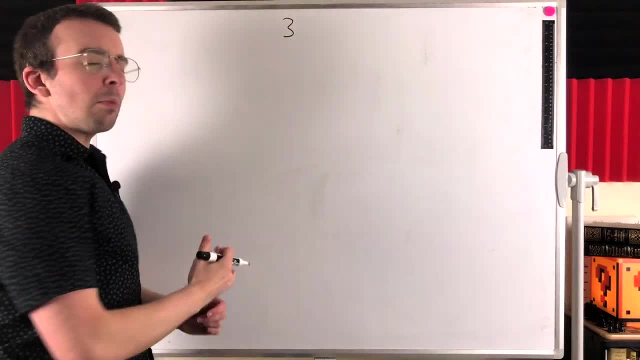 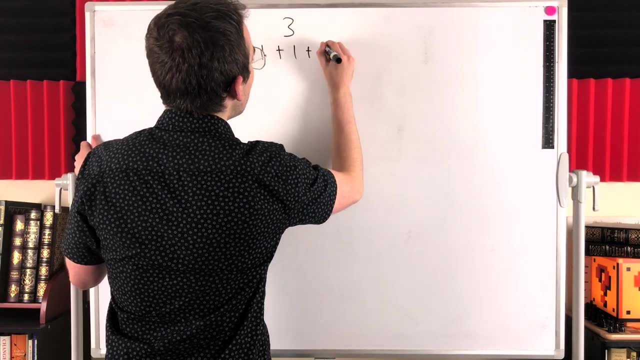 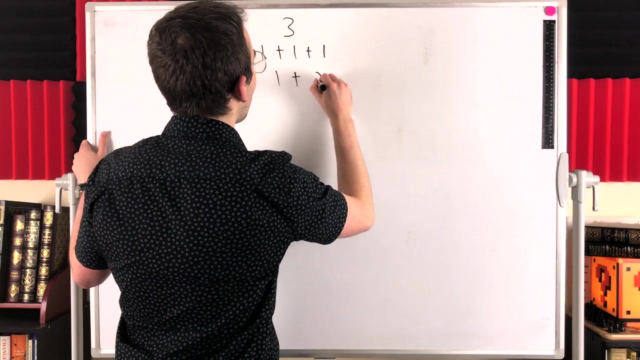 Positive integer 3, that's a pretty cool positive integer. How many ways can we write it? as an ordered sum of ones and twos? Well, certainly, for any positive integer n, we could write it as 1 plus 1 plus 1 n times. so that's one of the possibilities. For 3, we could also write it as: 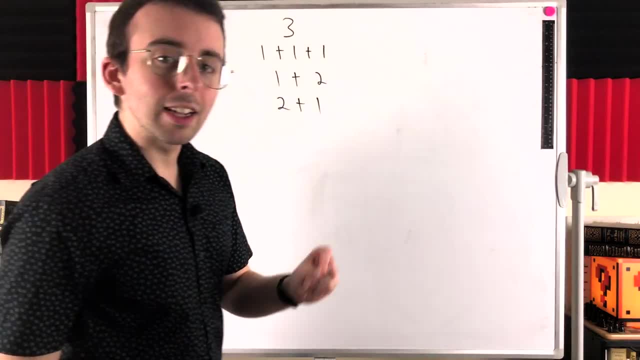 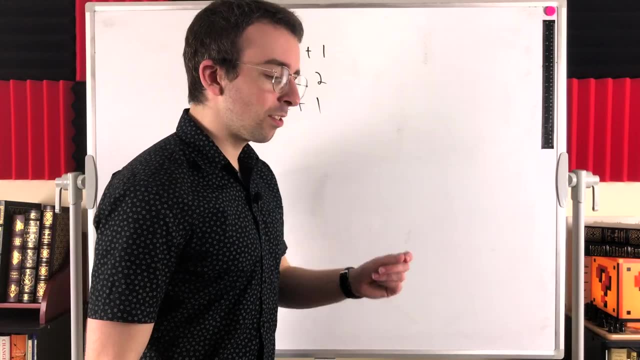 1 plus 2 or 2 plus 1.. Those are the three ways that we could write 3 as an ordered sum of ones and twos, And I apologize, this is going to be one of those lessons where I use the same. 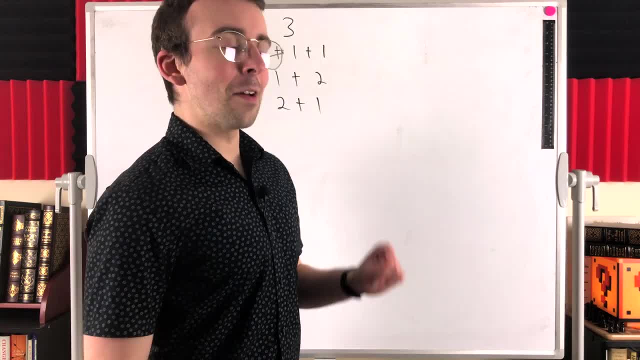 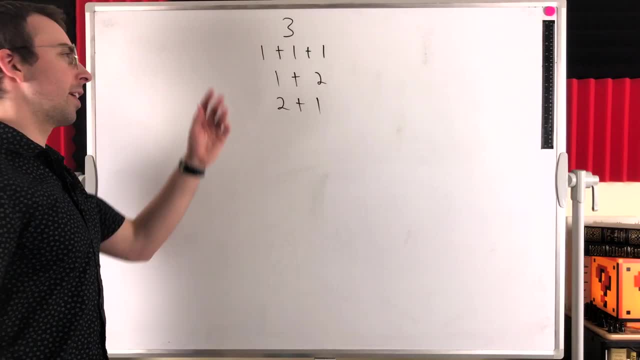 words over and over again. Usually it's the word set, but in today's lesson it's going to be sum 1, and 2.. We'll be using those words a lot, So here are the three ways we could write 3s. 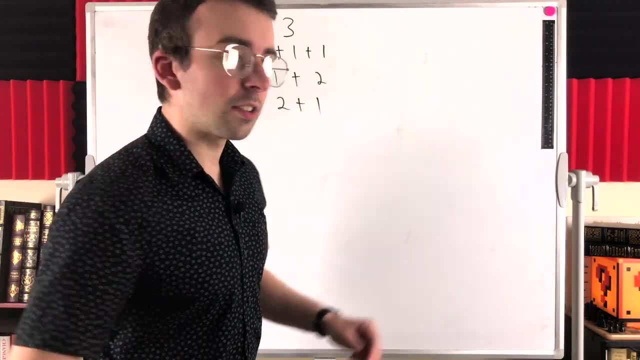 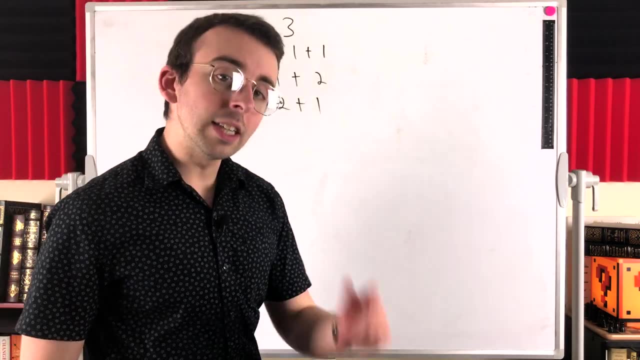 an ordered sum of ones and twos. Note that we're counting ordered sums, so we count 1 plus 2 and 2 plus 1 separately, because even though the sums have the same terms, they're in a different order. we're counting ordered sums. 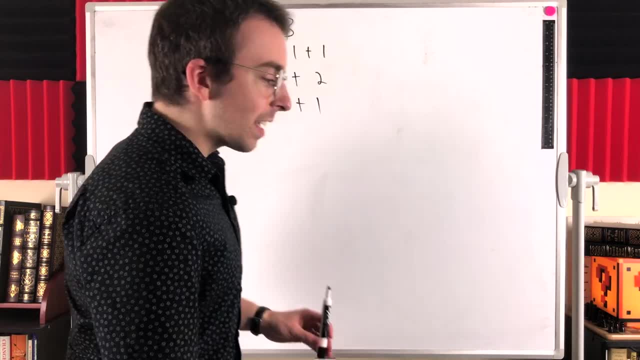 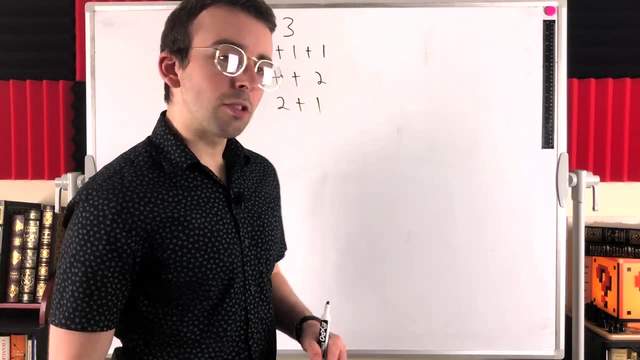 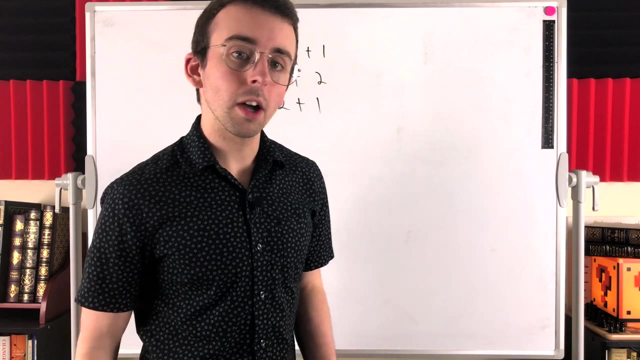 Okay, so how are we going to solve the problem in general, given any positive integer n, how many ways can we write it as these sorts of sums? What's going to help us answer this question is by thinking of each term in the sum as a possible position where we could put a 1. 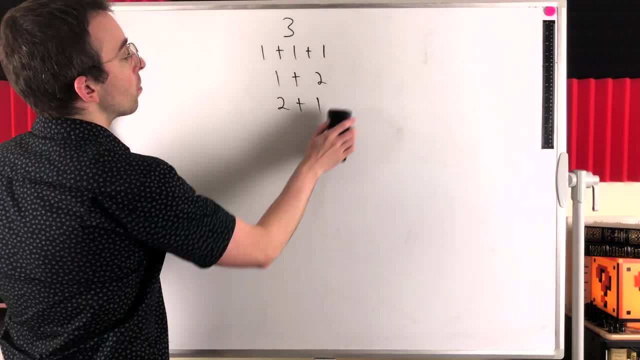 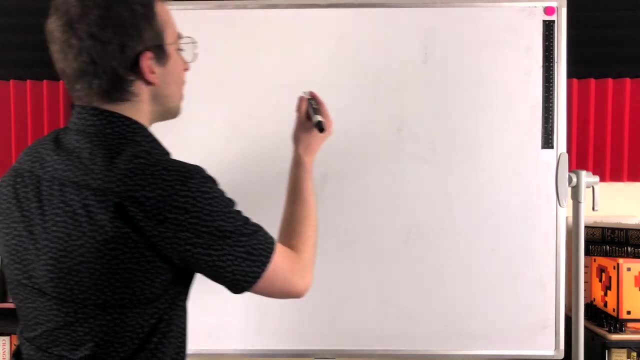 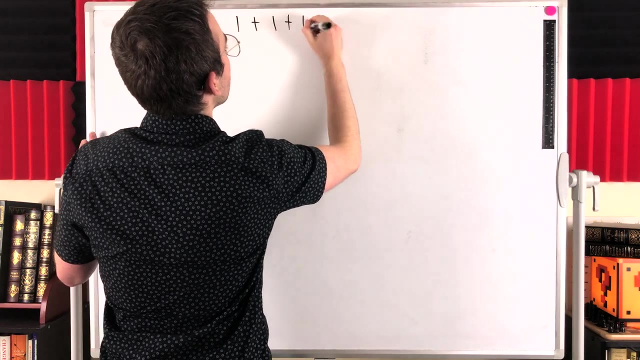 or a 2.. And we want to start from that really basic sum of 1 plus 1 plus 1, and so on. So let's begin explaining the general solution. Like we said, any positive integer n, we can certainly write it as 1 plus 1 plus 1, and so on. n times That will. 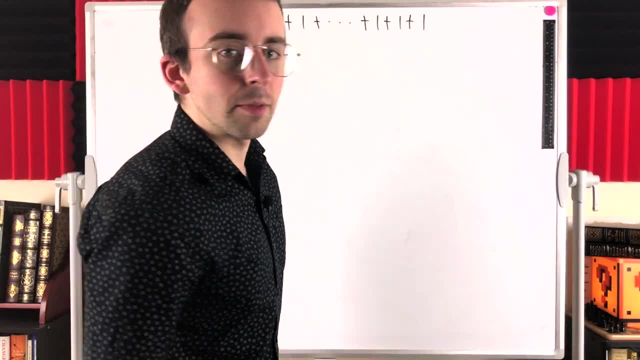 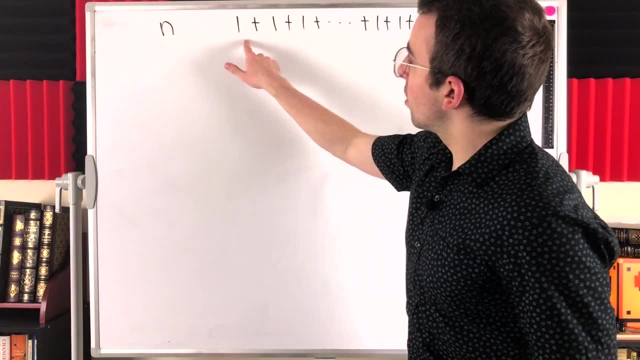 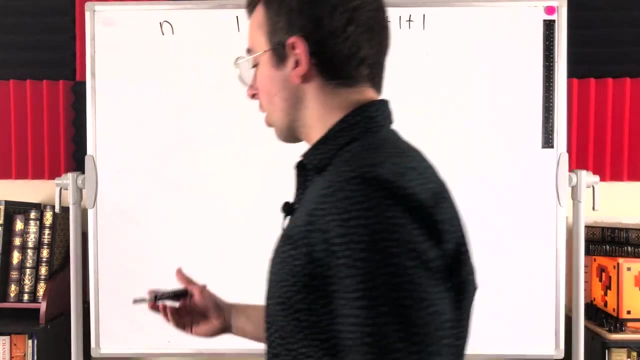 certainly give us one way of writing any positive integer n. We can just add a bunch of 1s together. One way to think about this is that there are n positions in this sum. right, Because there are n copies of 1, we can think of each term in the sum as being a position. So one way to kind of 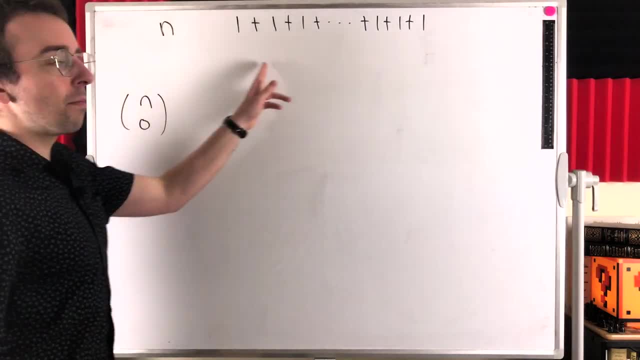 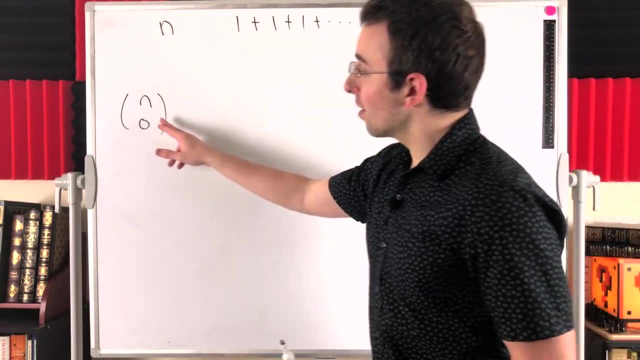 write n is n choose 0. There are n positions in the sum, and we're choosing 0 of them to be equal to 2.. And so this tells us: n choose 0, that's equal to 1.. And so that means there's one way. 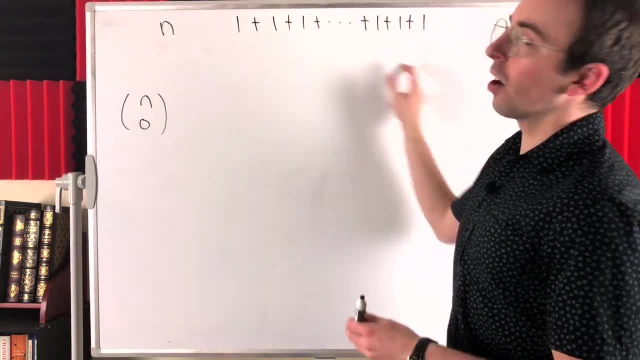 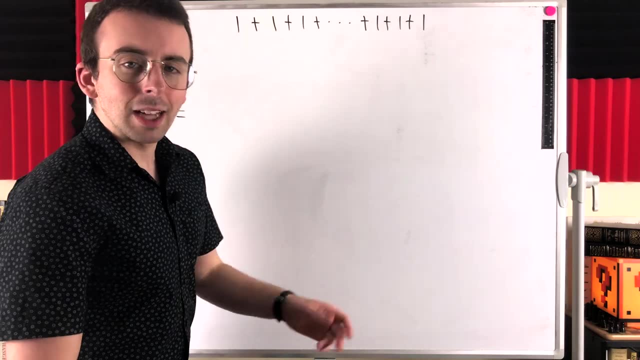 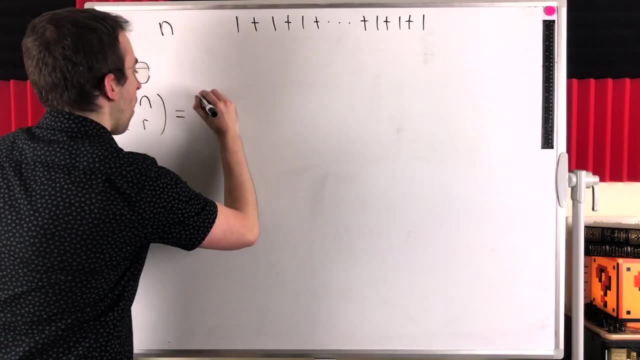 that we could write n as a sum of just 1s. Pretty straightforward. Remember, this is a binomial coefficient. I'll leave a link in the description to some lessons I have on binomial coefficients, But quickly, if you're not familiar with them, this is read: n choose r and it's equal to n- factorial. 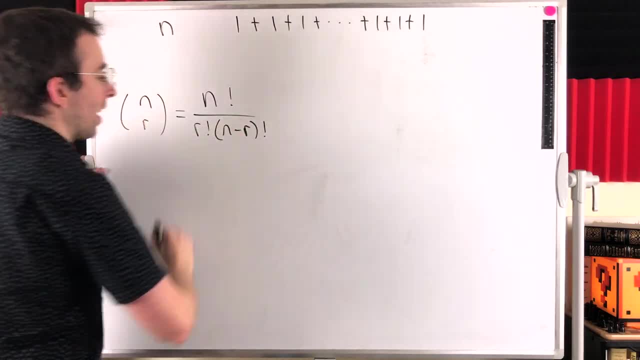 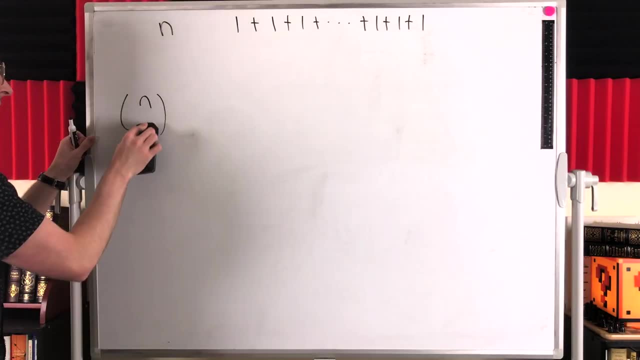 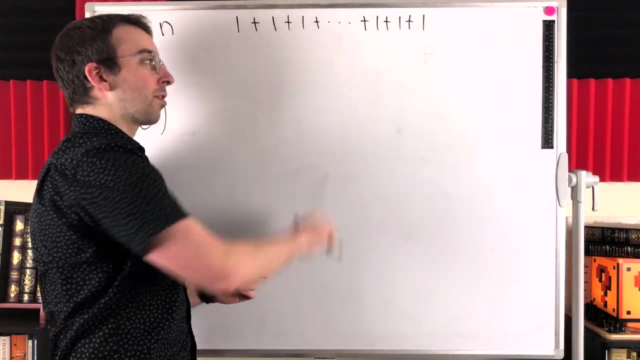 divided by r factorial times: n minus r factorial. But really, to get the most out of this lesson, you should probably already be familiar with this. Alright, so n choose 0, blahdy, blahdy, blah. There's one way we can write a positive integer as an ordered sum of just 1s. 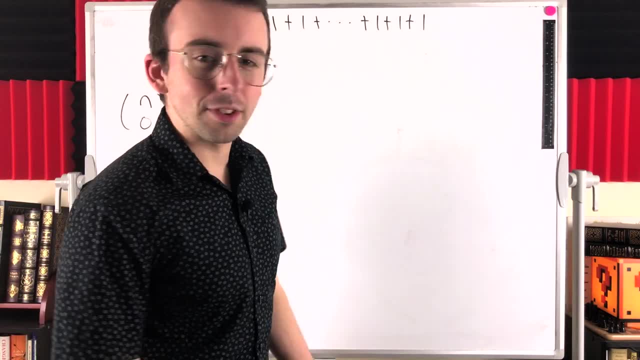 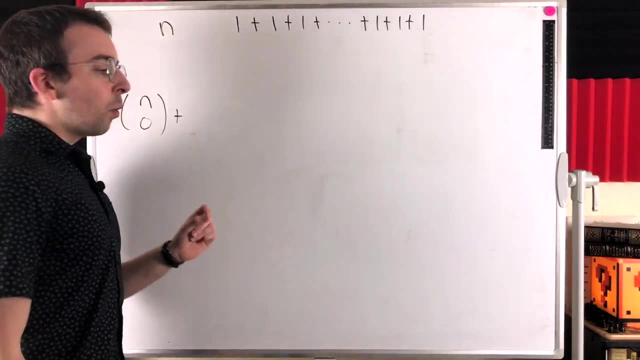 right. There's no way we can change the order here, because all the terms are the same. So then what if we want to include a 2 in the sum, because that's another possibility? Well, if we want to include one copy of 2 in the sum, we're going to have to get rid of 2 of the. 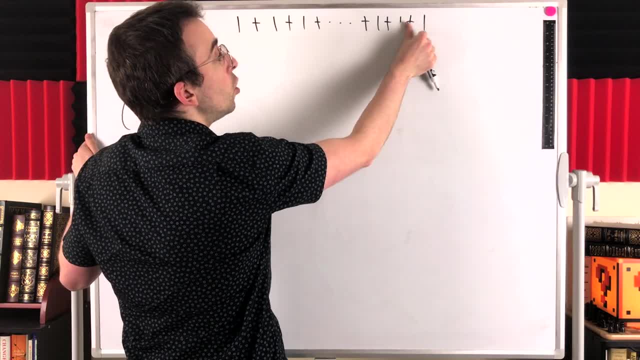 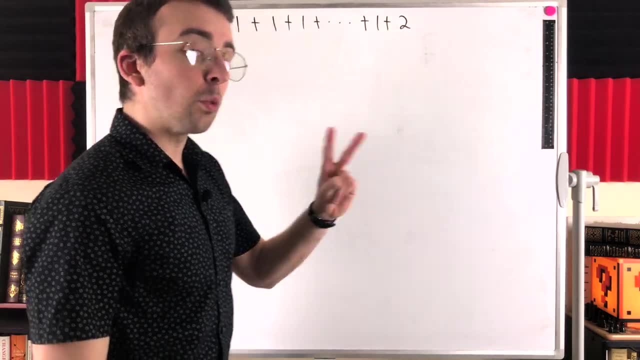 current positions. in the sum We're going to have to get rid of 2 copies of 1, so that the sum is still equal to the same thing when we add that 2. So we lose 2 copies of 1, that's losing 2 positions. 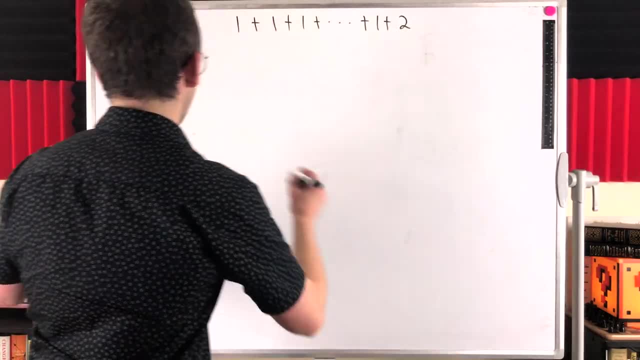 but we get 1 position back when we add that 2.. So we're going to have to get rid of 2 of the current positions in the sum. So now we originally had n positions. in our sum we lost 2 positions. 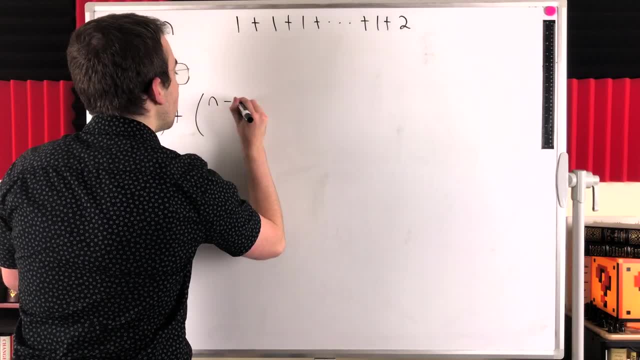 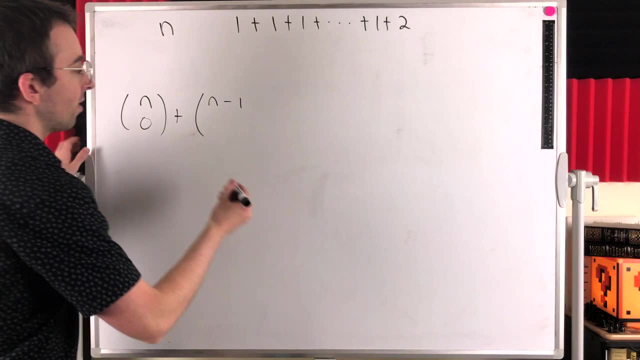 but got 1 position back. So now there are a total of n minus 1 positions And among those n minus 1 positions or terms in the sum, we can pick any one of them to be our copy of 2.. So you can see here. 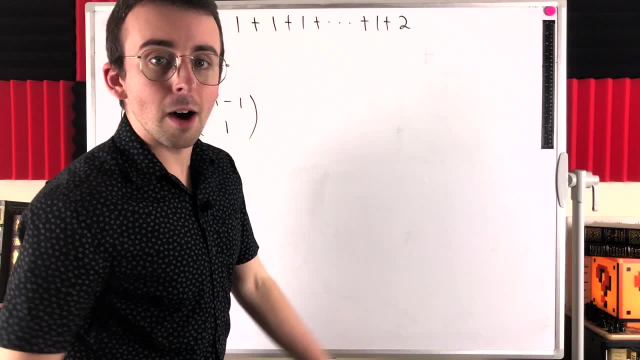 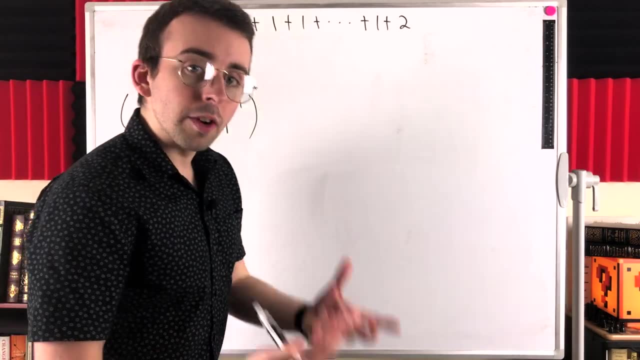 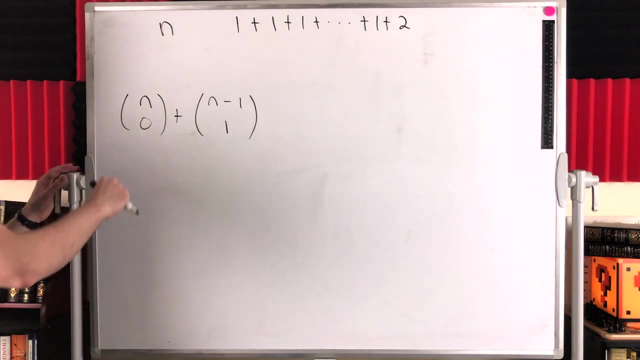 we're using these binomial coefficients, which count combinations, to count the number of ways we can order the sum for a given number of copies of 2 that are going to be in the sum. So for a positive integer n, there are n. choose 0, or 1 ways we can write it if we're. 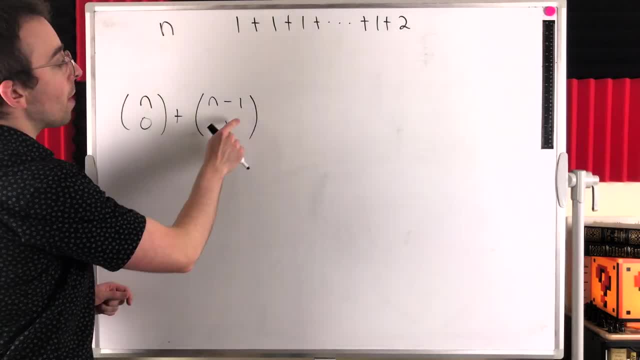 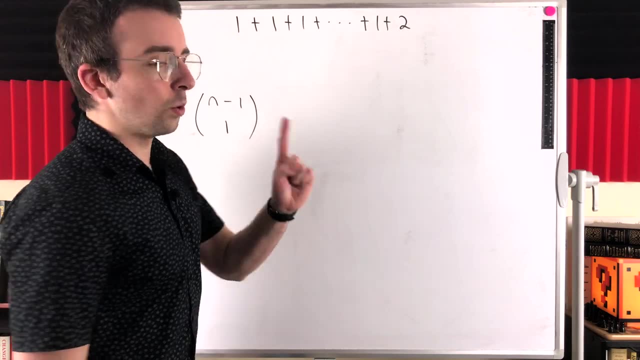 going to have 0 copies of 2.. And there are n minus 1. choose 1, or just n minus 1- ways to write it as an ordered sum of 1s and 2s if we're going to include 1 copy of 2.. And this pattern continues. 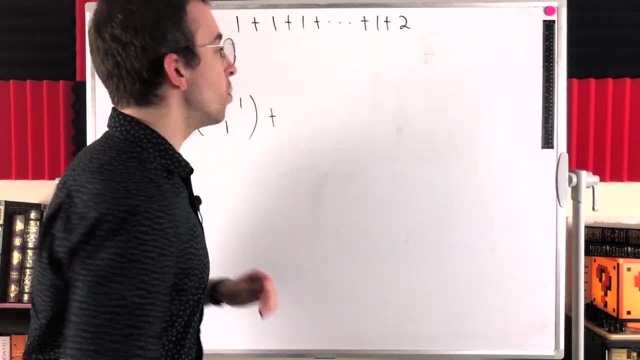 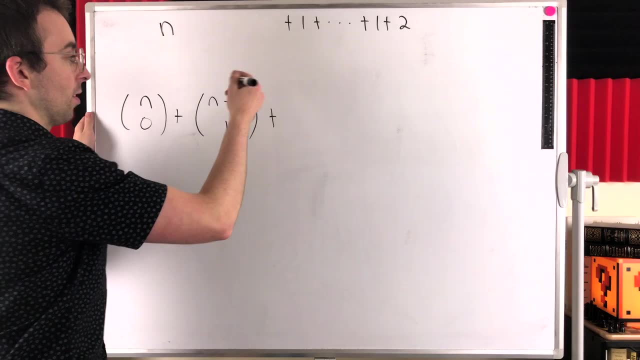 If we're going to include a second copy of 2 in the sum, then again we're going to have to get rid of 2 of the positions. we need to get rid of 2 of the 1 terms so that the sum is still equal to the. 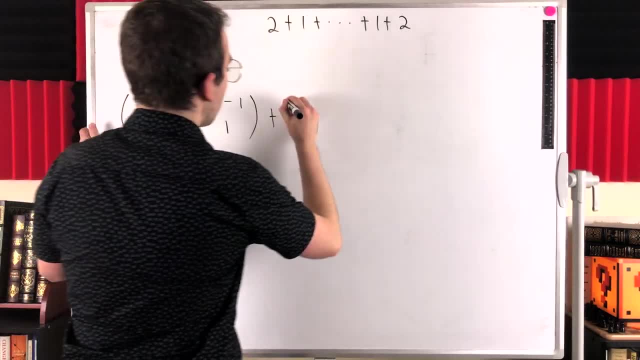 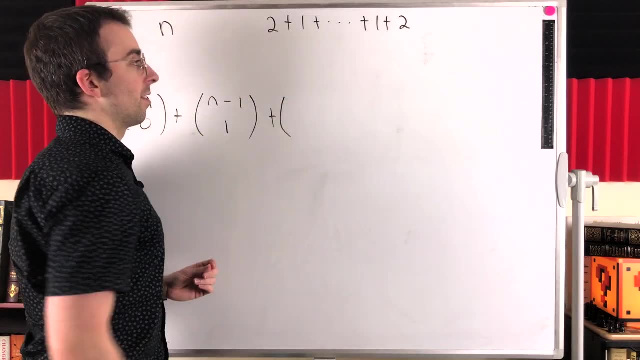 same thing once we add in another copy of 2.. So in total, every time we add a copy of 2, we have a net change of losing 1 position in the sum, because we lose 2 copies of 1, and we get that 1 copy of. 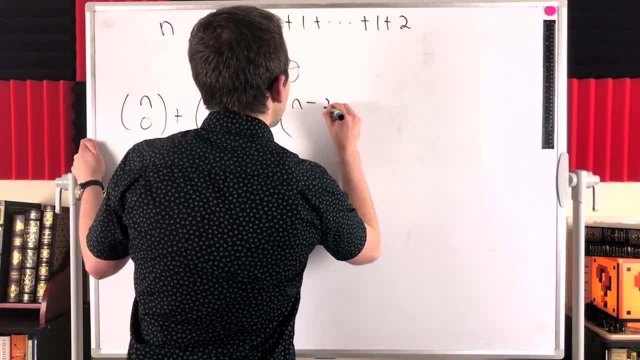 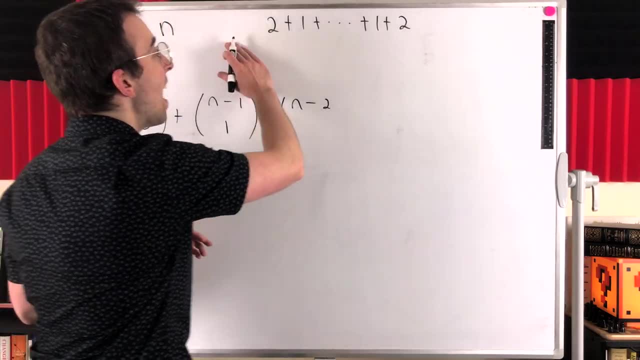 2 that we're adding. So if we add another copy of 2, we get a total of 1.. So if we add another copy of 2 into our sum, then we go from n minus 1 total positions to n minus 2 total positions. 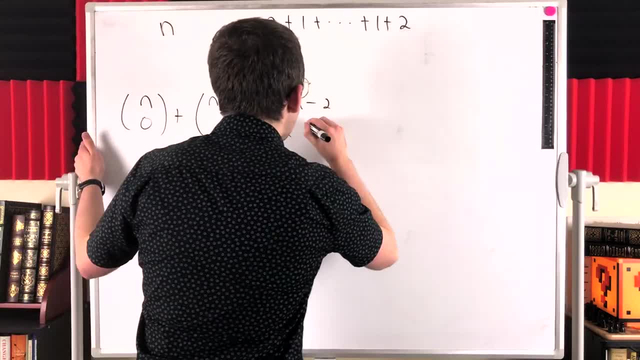 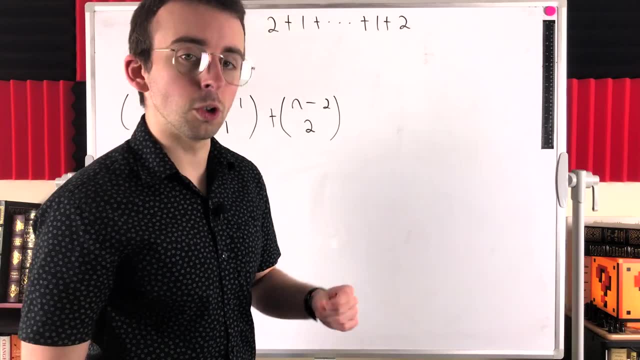 And of those n minus 2 total positions, we can pick any 2 of them to be our copies of 2.. So there are total of n minus 2. choose 2 ways that we could represent n as an ordered sum of 1s and. 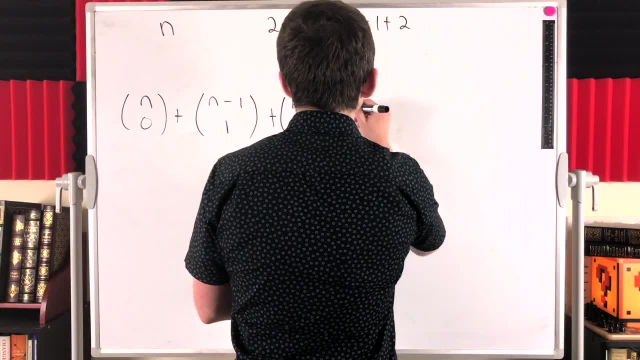 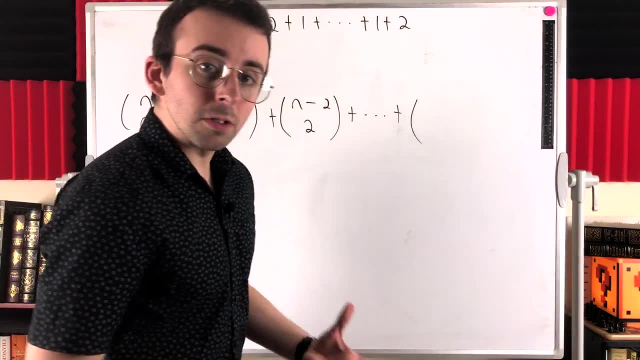 2s when we've got 2 copies of 2.. And so then we just continue in this way to get rid of 1, to count all the different ways that we could write n as an ordered sum of 1s and 2s for every. 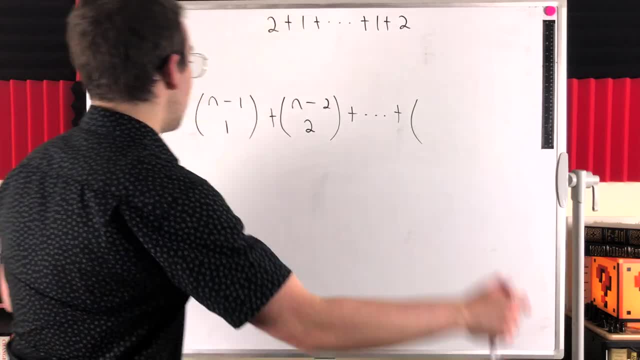 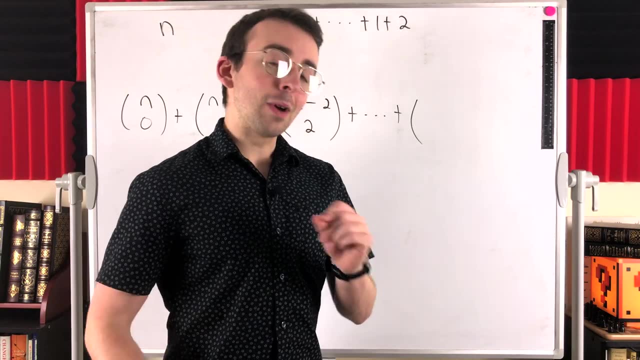 possible number of copies of 2 that it could have, going from 0 copies of 2 to 1 copy of 2 to 2 copies of 2, and so on. And so now the question just becomes: where do we stop? What's the maximum? 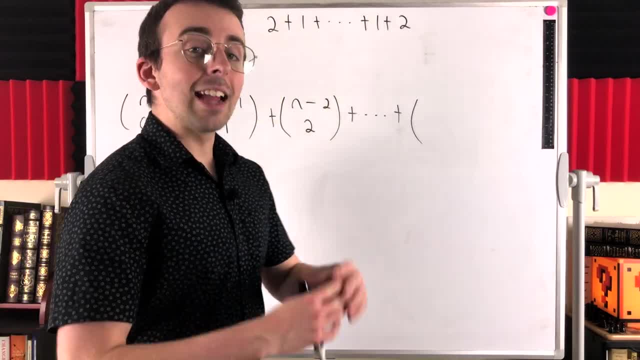 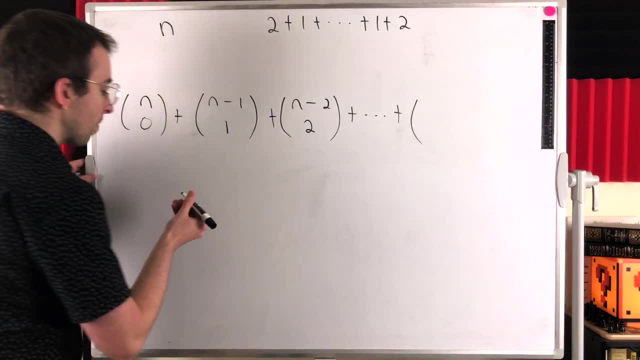 number of copies of 2 that we could have in a sum for a positive integer n. Well, that's pretty straightforward. if n is the maximum number of copies of 2 that we could have in a sum for a positive integer n, If n is, even then, certainly the maximum number of copies of 2 that we could, 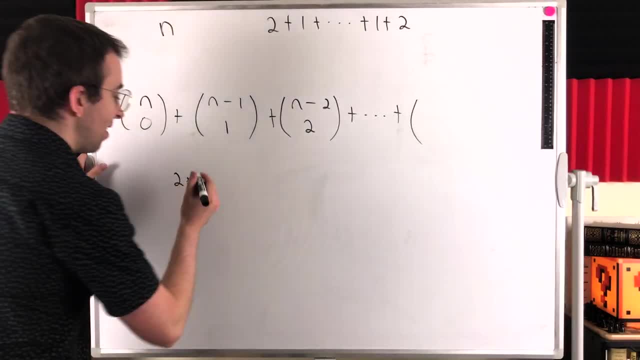 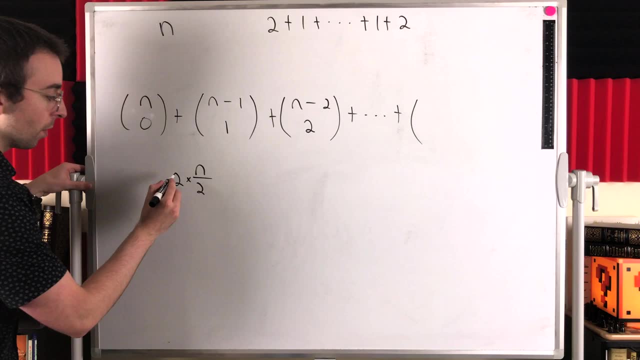 have in a sum that equals n. if n is even the maximum number of copies of 2 we could have in a sum is n over 2 copies of 2. Because of course the 2s cancel out and the sum would be equal. 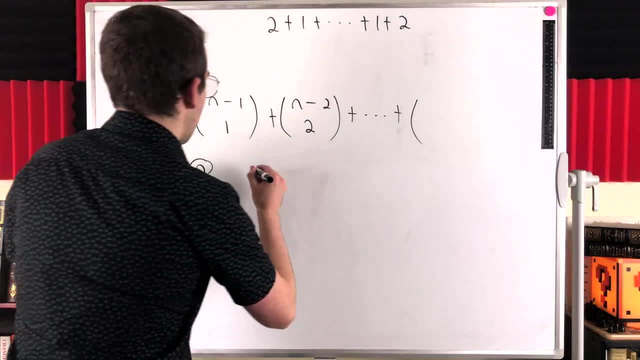 to the number n that we want. For example, if n was an even number like 4,, 4 over 2 is equal to 2, and so the maximum number of copies of 2 that we could have in a sum that equals n is n over 2.. 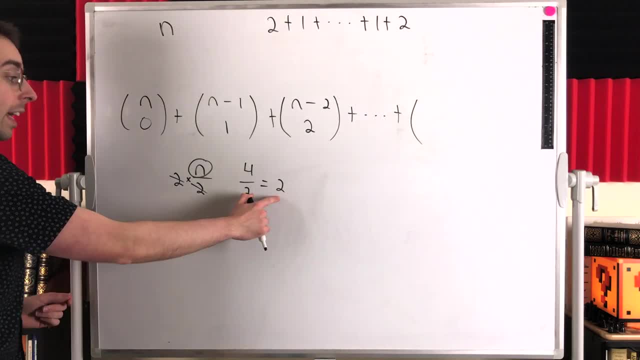 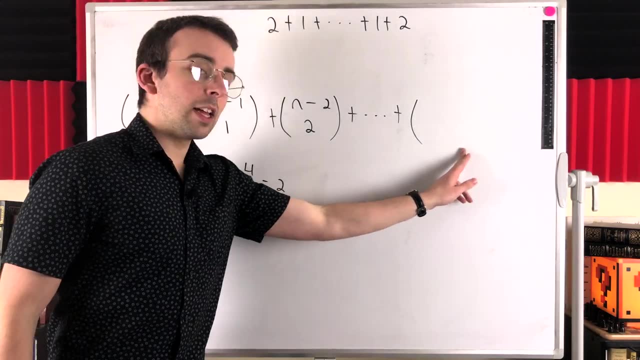 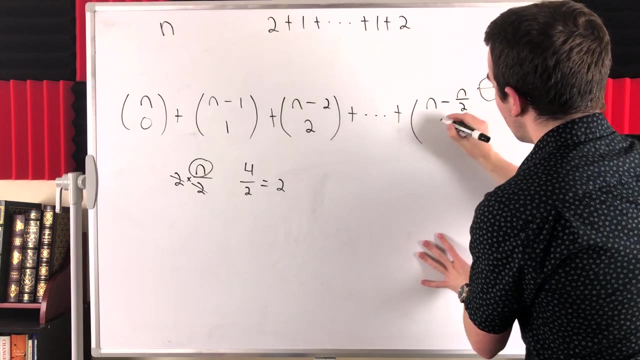 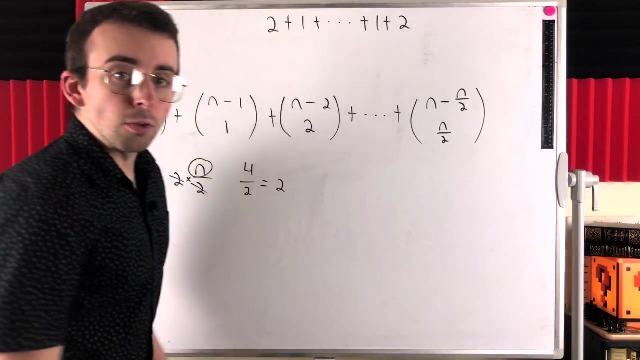 So if we're just concerned with even numbers at the moment, our sum would stop at our positive integer n minus half of n- choose half of n. So we would have n minus 0 plus n minus 1,- choose 1, plus n minus 2,- choose 2, plus n minus 3,- choose 3, and so on. 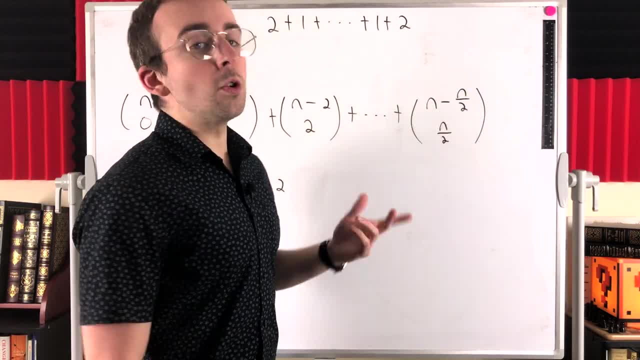 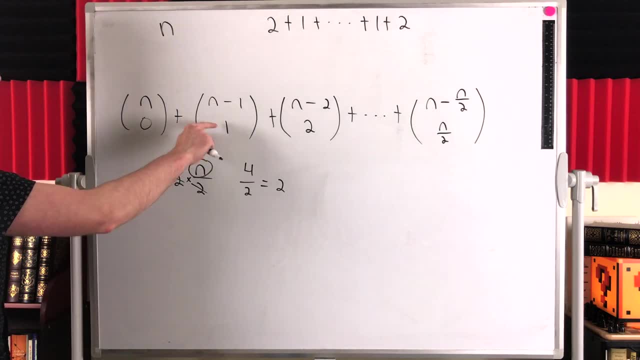 All the way up to n minus half of n. choose half of n. So for the number 14,, for example, it would be 14, choose 0, plus 13,. choose 1, plus 12,, choose 2,, and so on all the way up to 14. 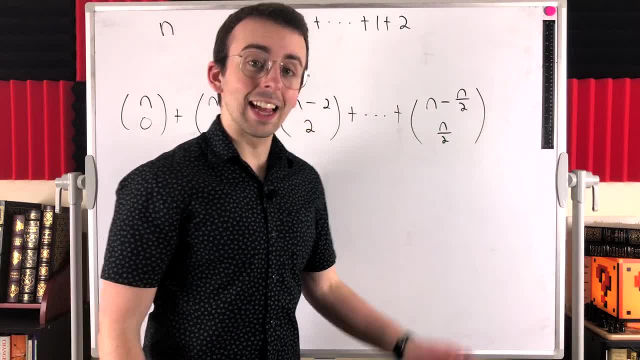 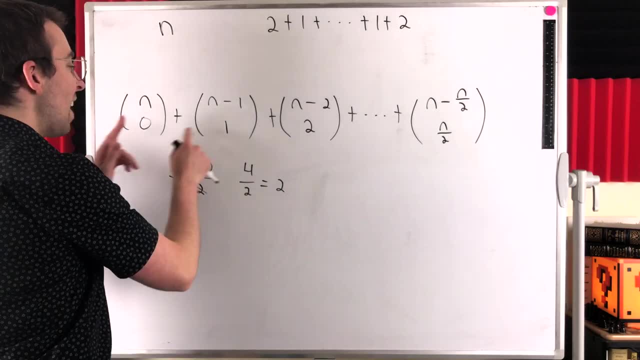 minus 7, which is 7, choose 7. And that's where the sum would stop. That would count all possible ways. We could write 14 as an ordered sum of 1s and 2s and the different terms in this sum. are 7 and 7.. So we could write 14 as an ordered sum of 1s and 2s, and the different terms in this sum are 7 and 7.. So we could write 14 as an ordered sum of 1s and 2s and the different terms in this. 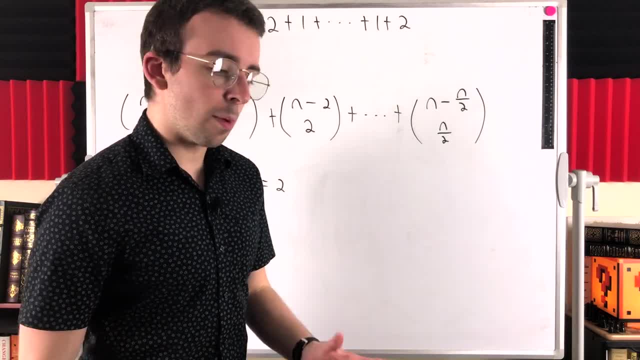 sum are 7 and 7.. So we could write 14 as an ordered sum of 1s and 2s and the different counting the number of ways that we could write it as a sum for different numbers of 2 that are: 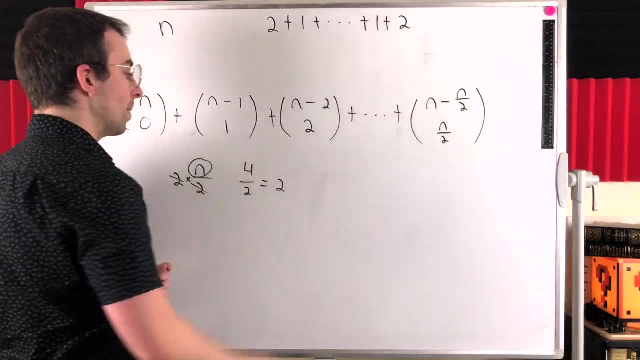 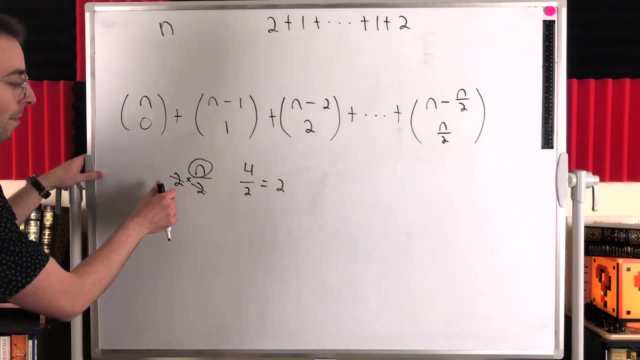 going to be in the sum for different numbers of copies of 2.. So then, what can we do to this solution, to adapt it for odd numbers as well? Well, if our number n is odd, then of course we're going to have a bit of a problem, a little bit of trickiness going on here. 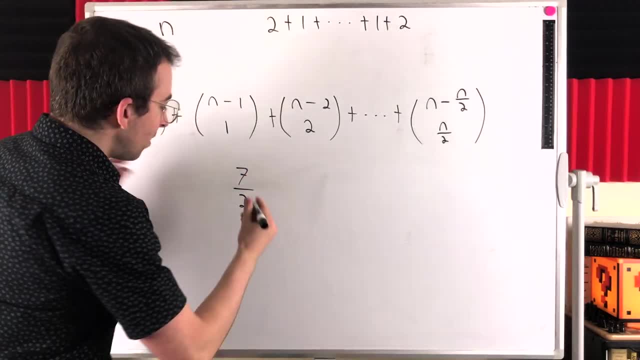 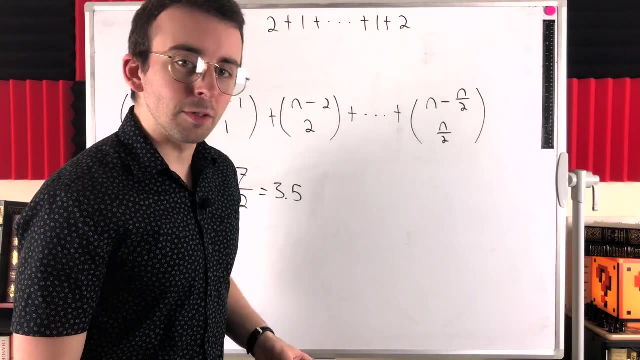 If we have the number 7,, for example, 7 over 2 is 3, and a half, and we can't really have 3 and a half copies of 2. in our sum, We can only have 2s and 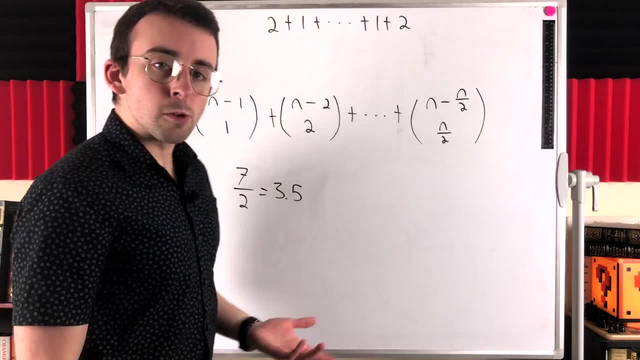 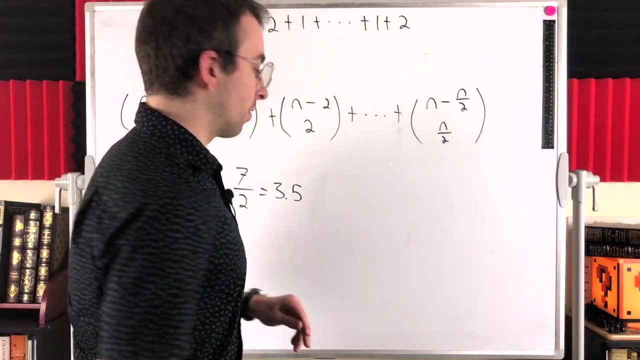 1s. So we might say: okay, well then we got to round 3 and a half. We either have to round it up or we have to round it down, and that's where we'll stop at that number of 2s If we round it up. 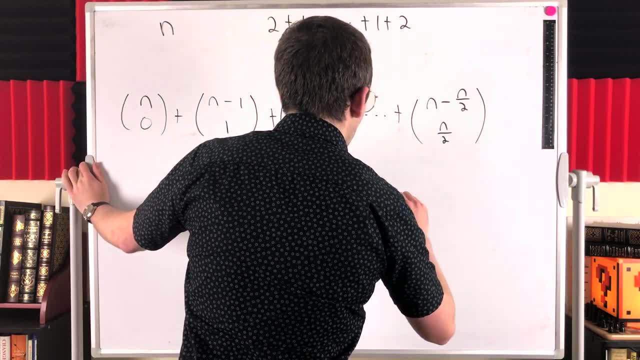 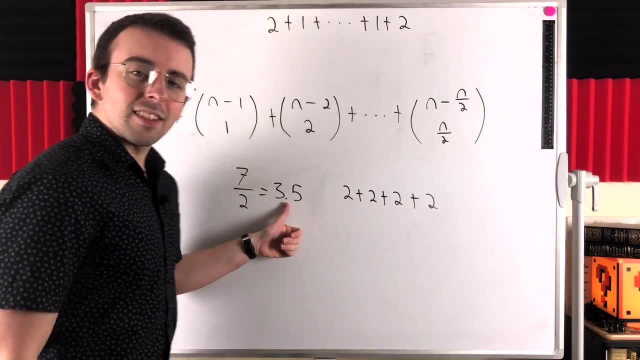 then we would have 4 copies of 2, and we would try to write 7 as an ordered sum of 1s and 2s, including 4 copies of 2.. But since we rounded this up, that's too many. That's equal to 8.. So then we'd have to subtract 1,. 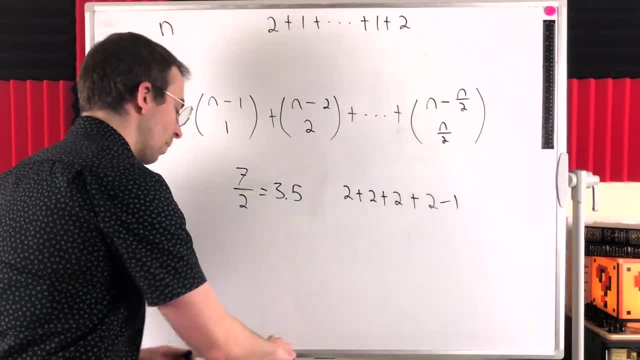 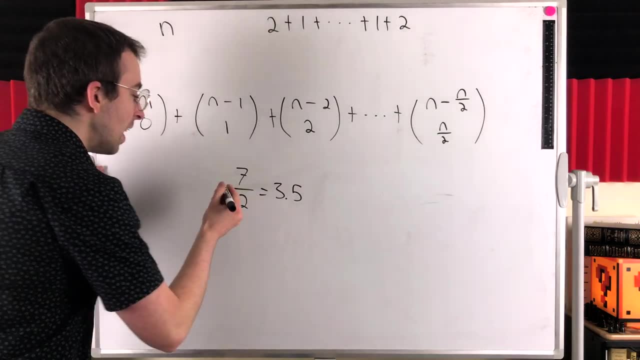 but that's not allowed, because we're just adding 1s and 2s. We can't do any subtraction, So we have to round down. We have to round down and, using some nice notation, we can use what's called the Floor Function. A lot of you are probably familiar with the Floor Function. 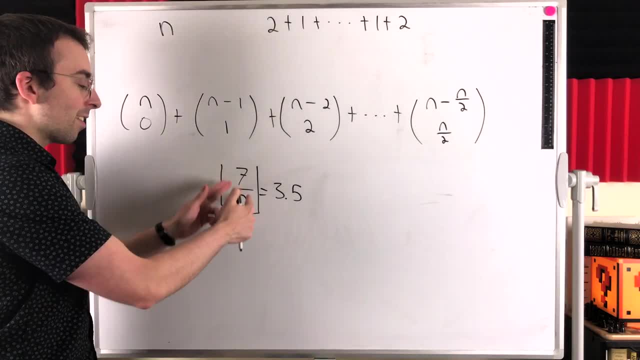 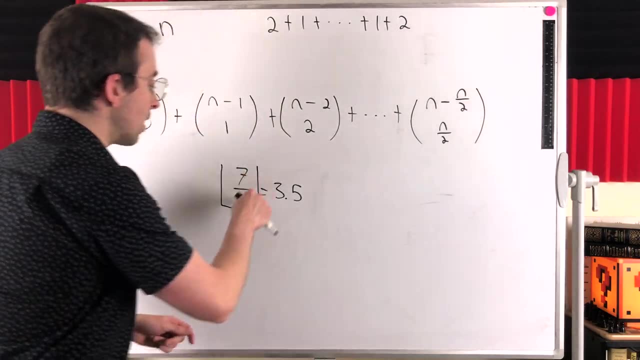 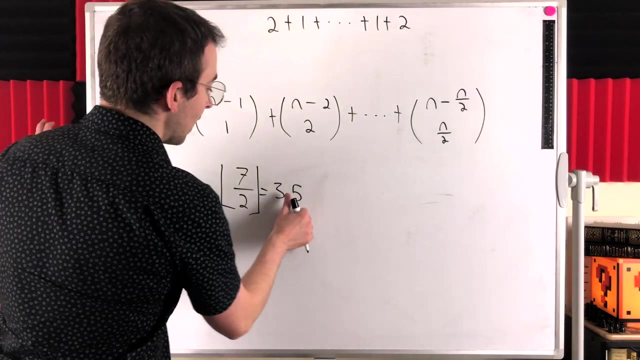 Some of you might not be. All it is is it takes the number inside of the function, in this case 7 over 2, and it spits out the nearest integer less than or equal to what's inside. So the nearest integer that's less than or equal to 3 and a half is 3.. 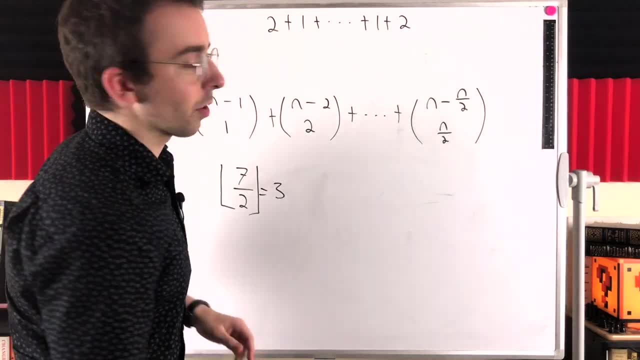 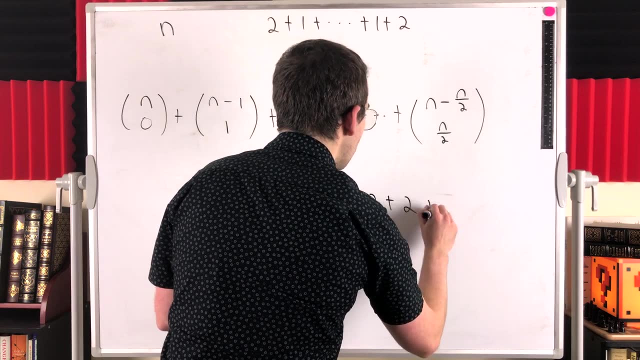 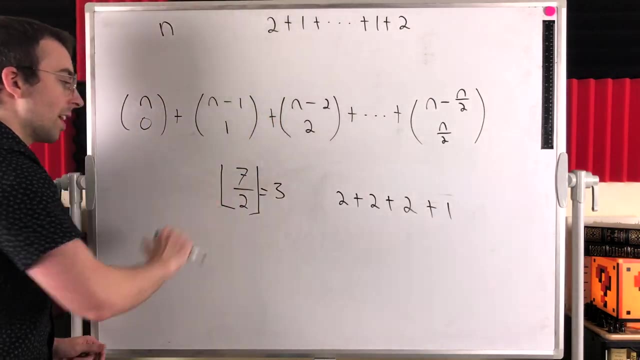 So the floor of 7 over 2, just 7 over 2, rounded down, is equal to 3.. So we would stop at a maximum number of copies of 2 of 3.. That's as many copies of 2 as we could possibly have in one of these ordered sums. that's going to be equal to 6.. 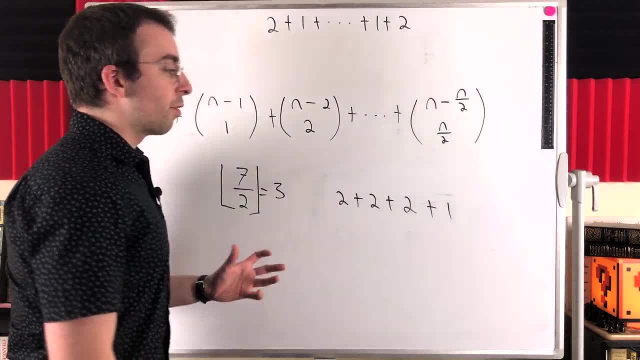 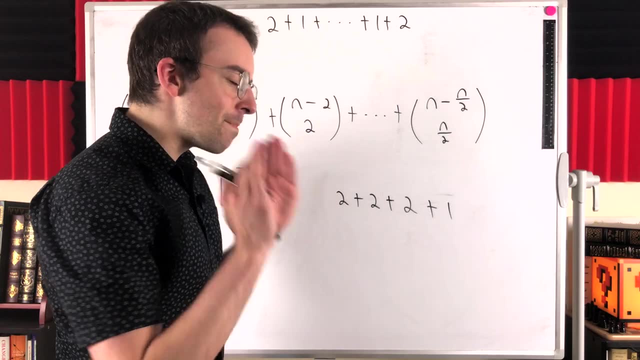 So that's what we have to do with the odd numbers. We have to divide them by 2 and round down, and that's where this sum would stop. for odd numbers, That's the maximum number of copies of 2 we could have. 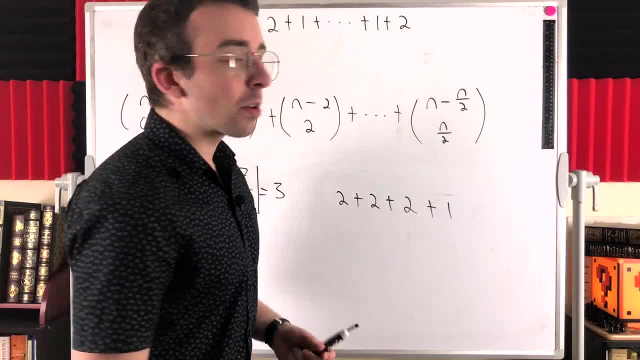 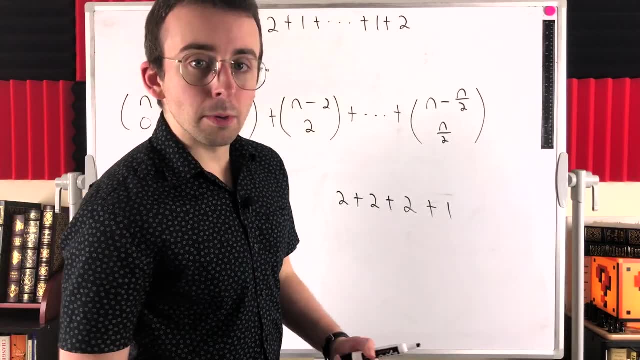 One more time. for an even number, the maximum number of copies of 2 we could have in our sum is half of the number. and for an odd number, the maximum number of copies of 2 we could have is half the number rounded down. 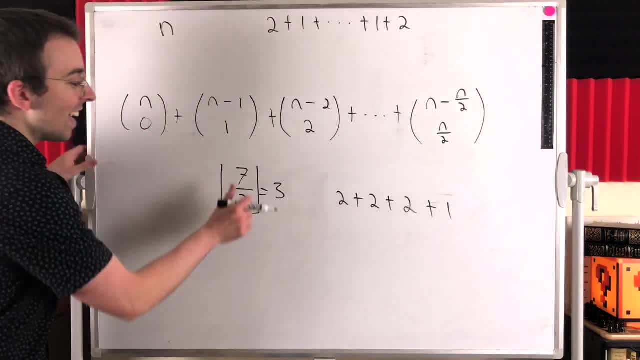 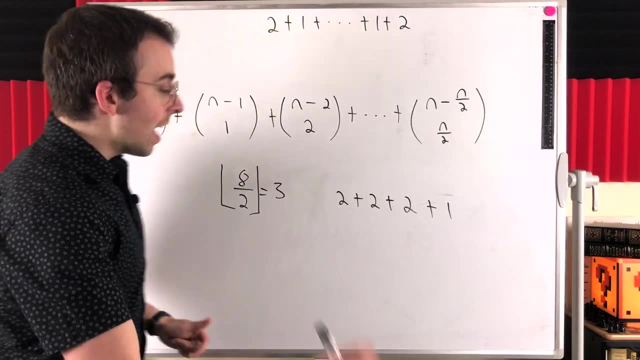 down Now. the very nice thing is that for an even number like 8, for example, 8 over 2 is equal to 4.. If we plug that into the floor function, the nearest integer less than or equal to 4 is just. 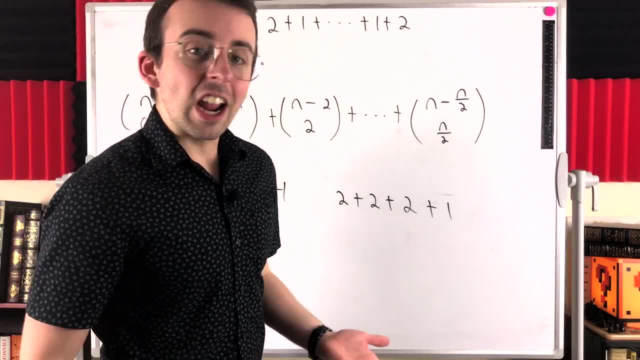 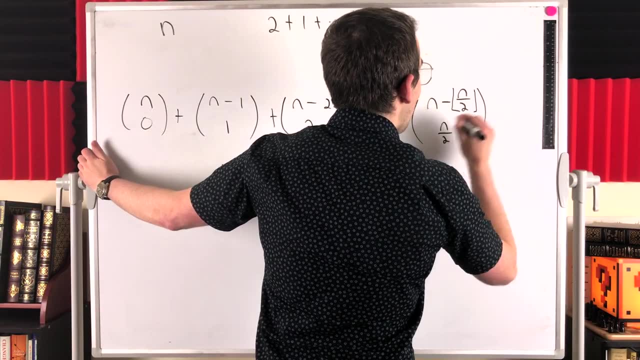 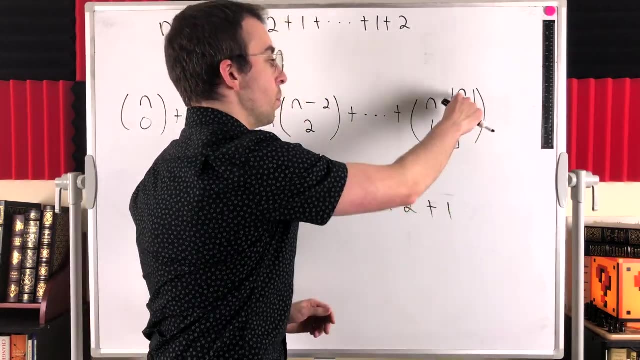 4. In other words, the floor function doesn't change the value of an integer. So we can apply the floor function in all cases, whether n is odd, or even If n is odd, the floor function is going to do what we need it to do to bring the decimal number down to a nice integer. And if 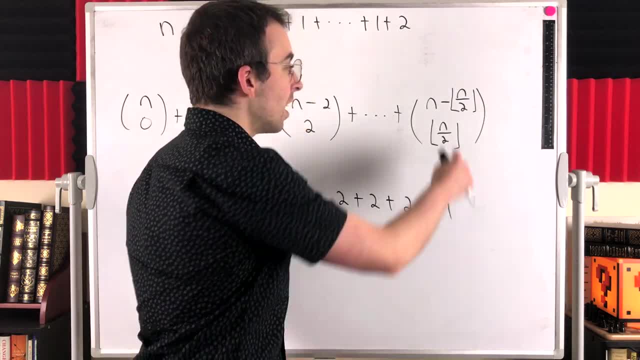 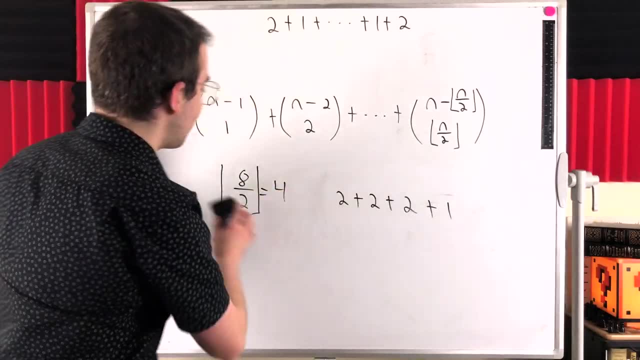 it's an even number, the floor function isn't going to change anything, because an even number divided by 2 is an integer, and so the floor function won't change it. And so, my friends, this is our solution Now, if we write it as a nice sum using summation notation. 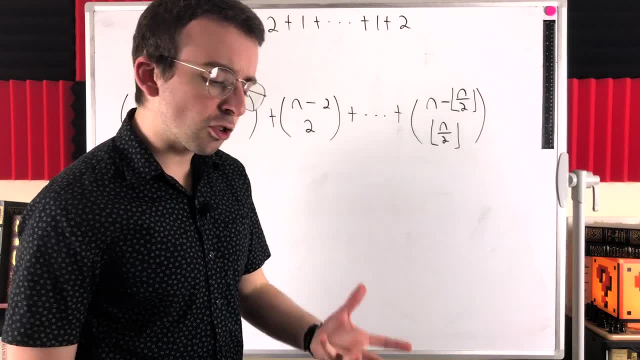 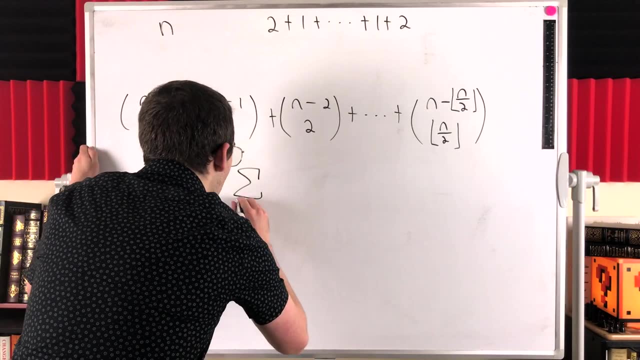 we're saying the total number of ways that we can write a positive integer n as an ordered sum of 1s and 2s is equal to this. It's equal to the sum from: i equals 0 to i equals the floor of n over 2,. 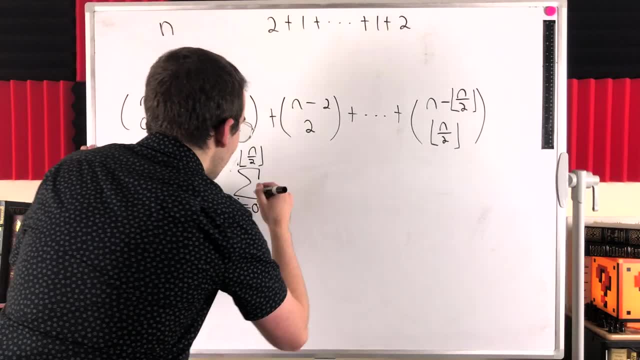 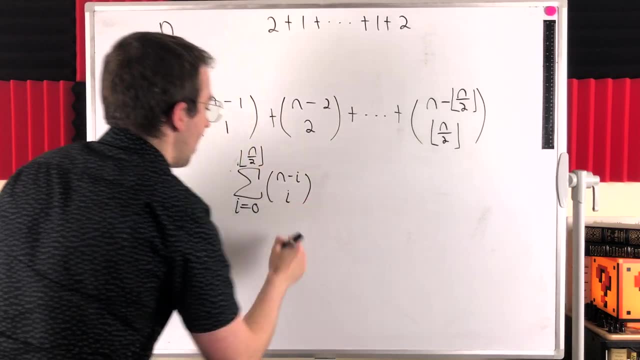 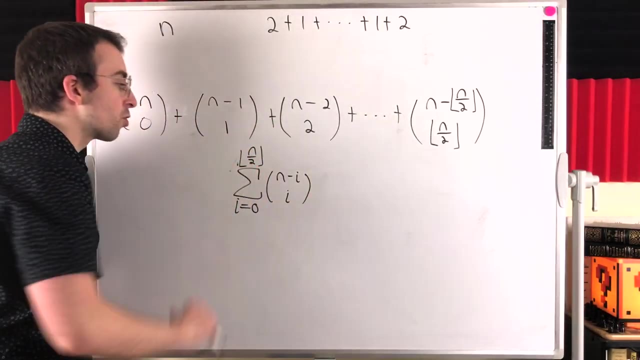 which is just half of n. rounded down, this sum from n- or it's the sum of n minus- i choose i from i- equals 0 to half of n rounded. That's the total number of ways we can write a positive integer n as an ordered sum of 1s and 2s. 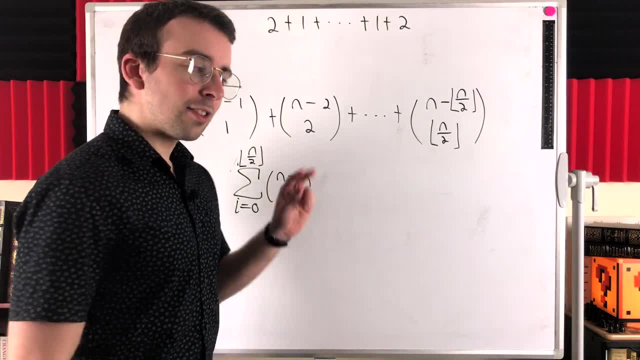 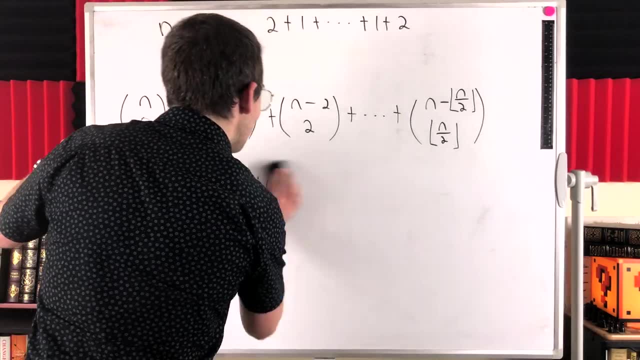 Pretty cool, fairly elegant solution. So let's check out a couple quick examples, and you'll find there's something rather surprising going on here that you certainly don't want to miss. So, once more, I just wrote the sum that we just explained here. 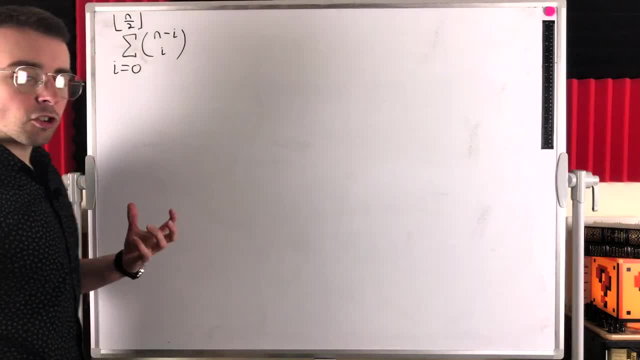 just for our nice handy reference. and remember that each term in this sum for a given value of i, for example, i equals 0 to i- is equal to the sum from: i equals 0 to i equals 0 to. i equals 0 to i equals. 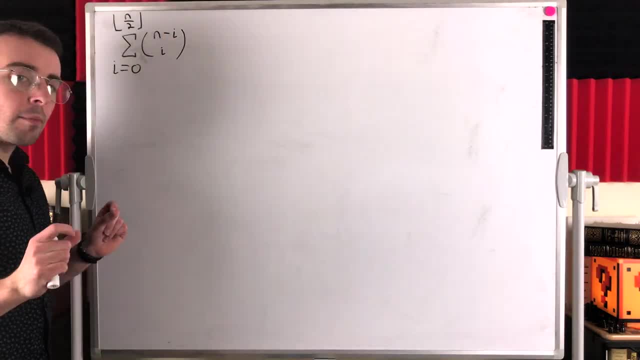 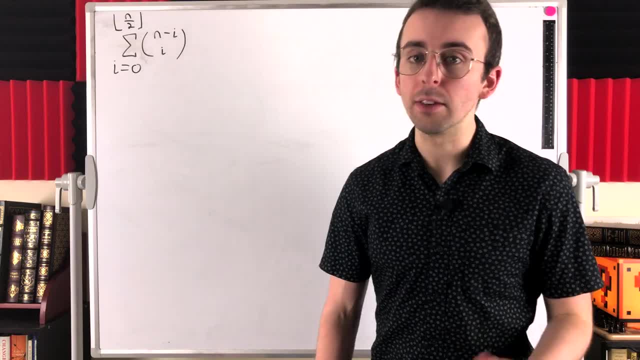 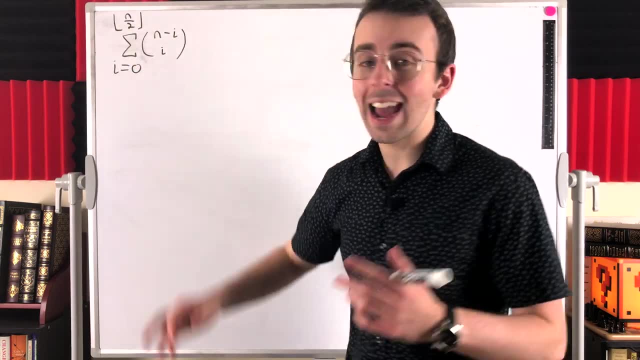 of 1s and 2s, where we have 3 copies of 2.. So each term in the sum is counting the number of ways we can write our number n using i copies of 2.. So for a few quick examples, how many ways can we? 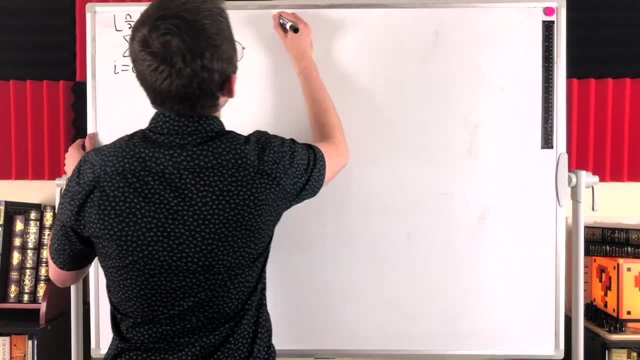 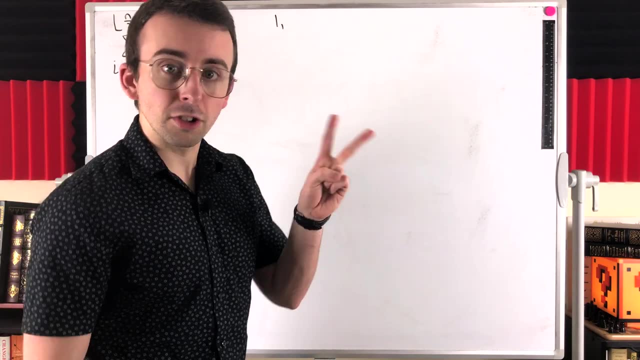 write 1 as an ordered sum of 1s and 2s. Well, there's only one way: we could just write it as 1.. How about 2?? We could write 2 as 1 plus 1, or just 2.. So there are 2 total ways: 1 plus 1 or 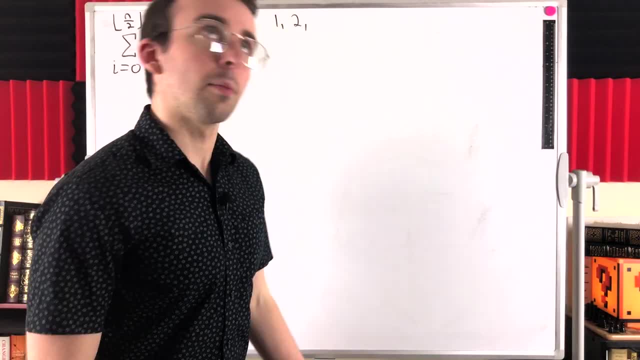 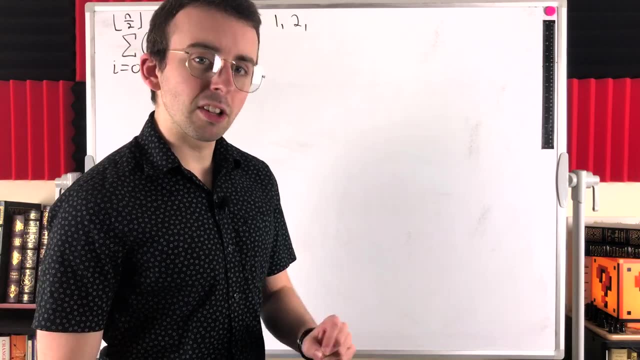 2. 2 ways we could write 2 as an ordered sum of 1s and 2s. How about the number 3?? Well, we saw at the beginning of the video that there are 3 ways we can write 3 as an ordered sum of 1s and 2s. 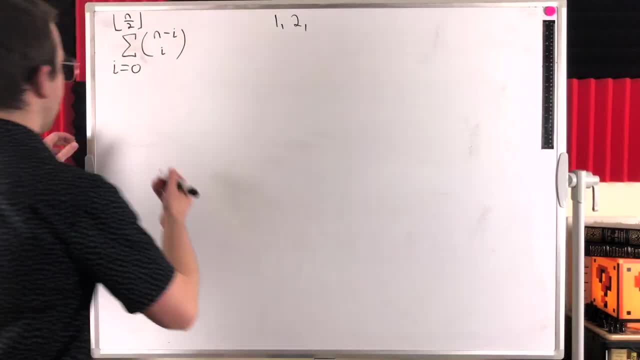 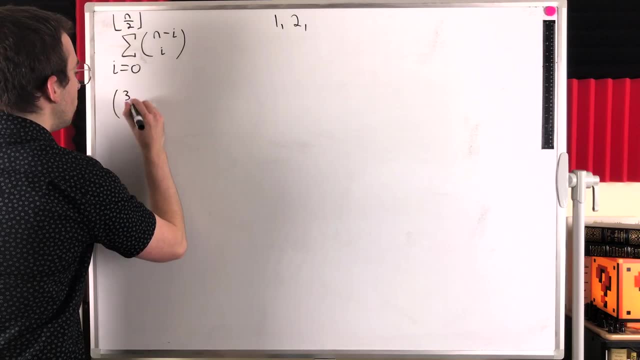 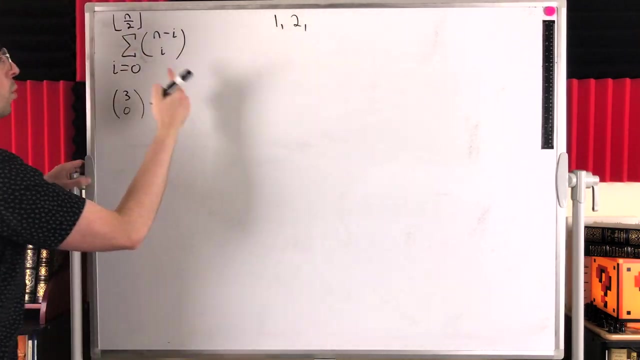 So let's just go ahead and try using our formula, see if we get the same answer. We would start at i equals 0, so that would be 3 minus 0- choose 0. and then we would increment up i by 1, so we would have 3 minus 1, which is 2 choose 1. 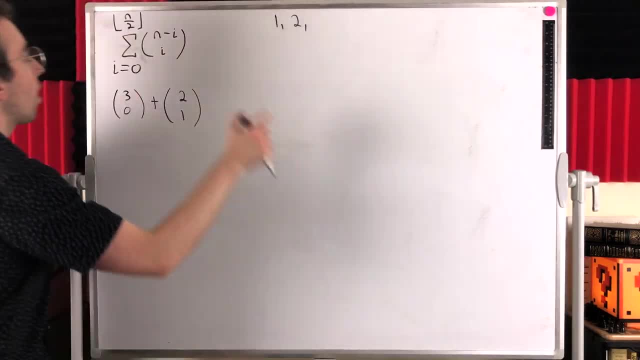 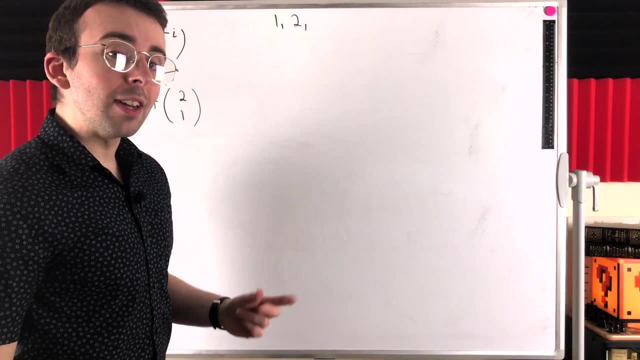 and then we want to keep our eye on where we have to stop. we have to stop at 3 over 2 rounded down. 3 over 2 is 1.5. rounded down with the floor function is 1. so we have to stop here where i. 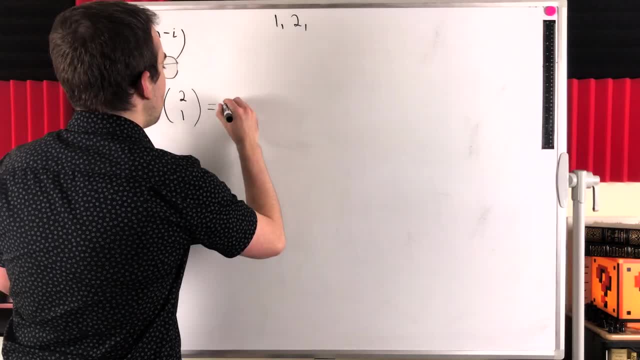 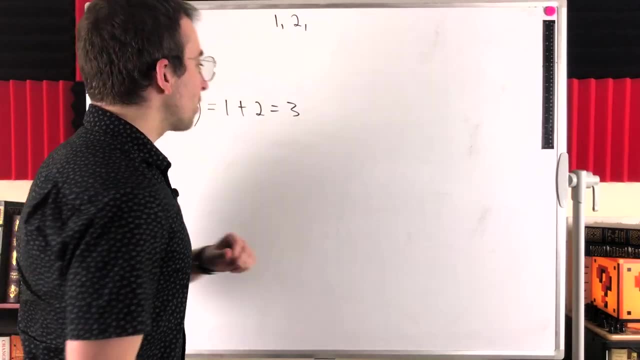 equals 1. what's this sum? equal to 3? choose 0 is 1, 2. choose 1 is 2. so it's 1 plus 2, which is 3, which is the same thing we saw earlier. so that looks good. so 3 is the next term in the sum, one more. 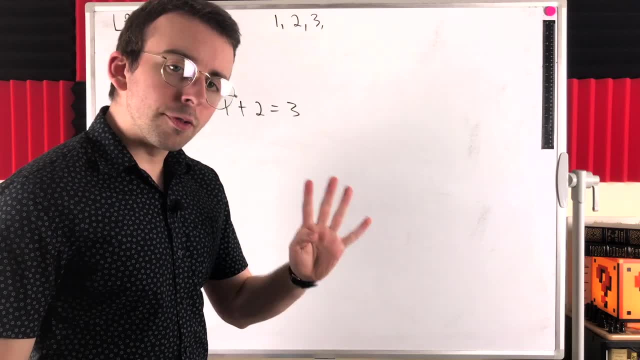 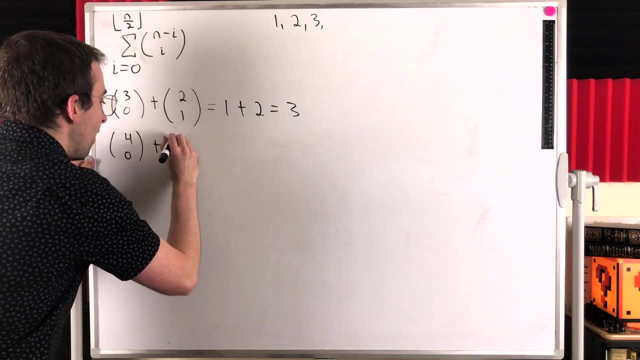 example, with our formula: how many ways can we write 4 as an ordered sum of 1's and 2's? well, we start with: i equals 0, so that's 4, choose 0, and then we just bring this number down: 1, this number. 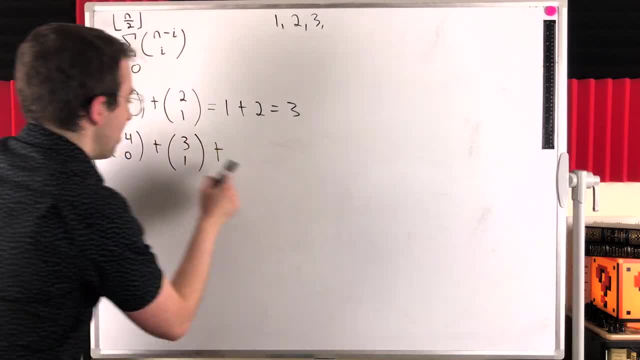 up 1, so 3 choose 0, and then we just bring this number down: 1, this number up 1, so 3 choose 0 and 2 choose 1, and then this number down: 1. this number up 1, 2 choose 2. we want to remember where. 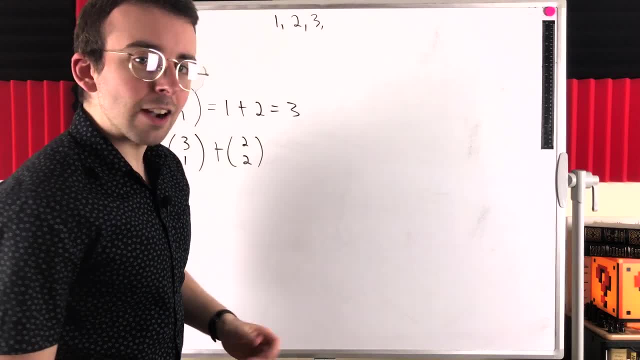 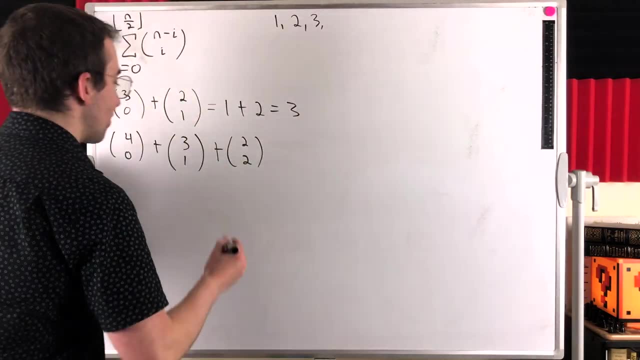 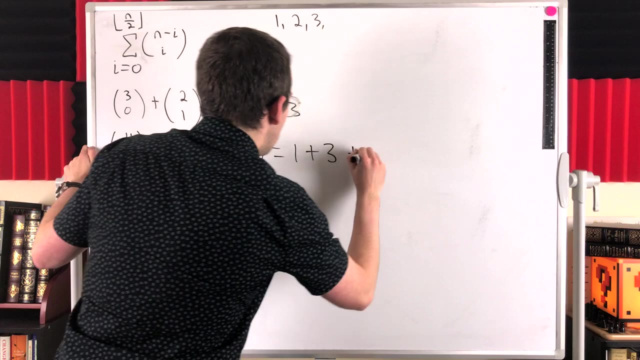 we have to stop. we have to stop at half of our number n. rounded down, half of 4 is 2. rounded down is 2, where i equals 2. so now we stop. what's this equal to 4? choose 0 is 1, 3. choose 1 is 3, 2, choose. 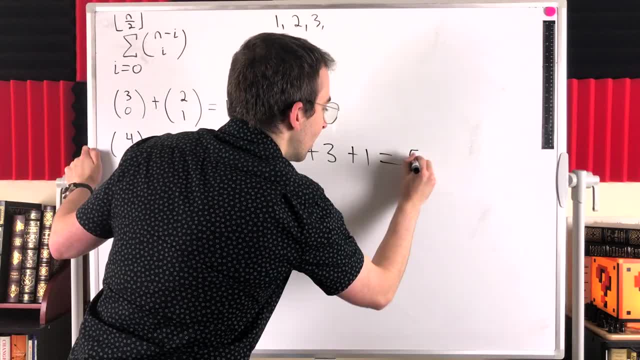 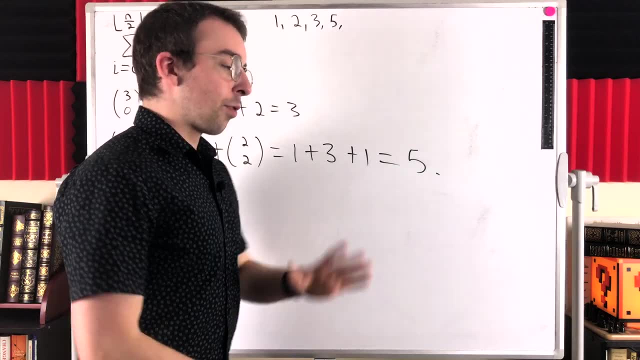 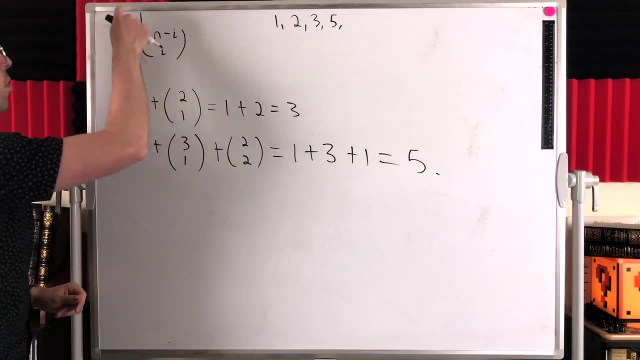 2 is 1, this is equal to 5. beautiful, all right, so i'll stop there. as our last example of applying the formula, for example, just to quickly mention it, the next number: 5. if we wanted to use this sum for the number 5, 5 over 2 is 2, and. 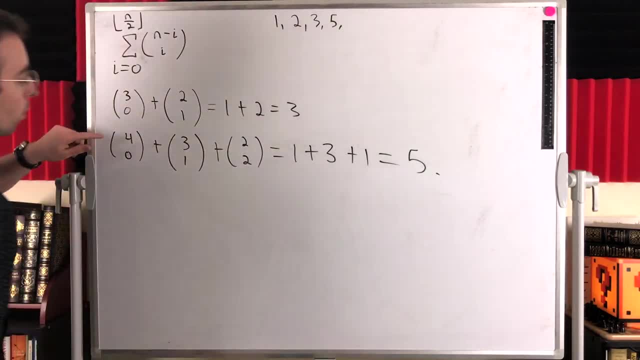 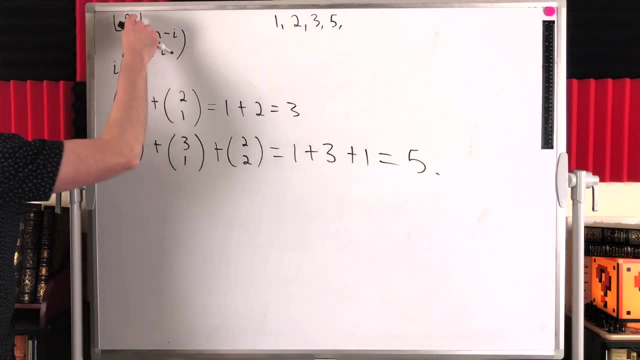 a half, rounded down is 2, so the sum would be 5- choose 0 plus 4, choose 1 plus 3, choose 2, and then we would stop there, at half of 5 rounded down, which is 2. the next few terms in this sum: 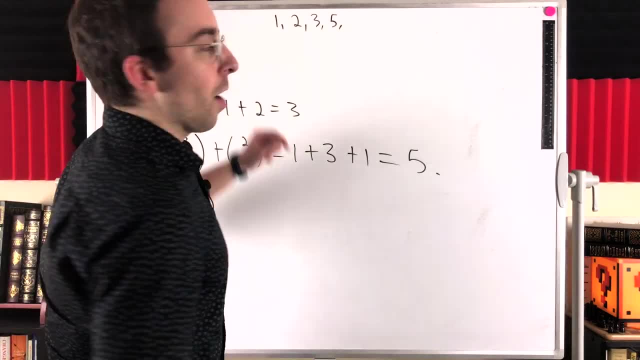 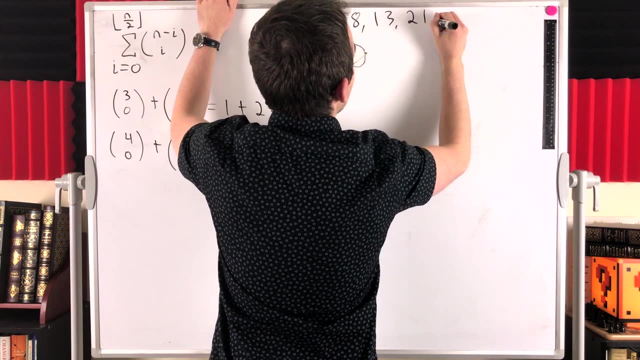 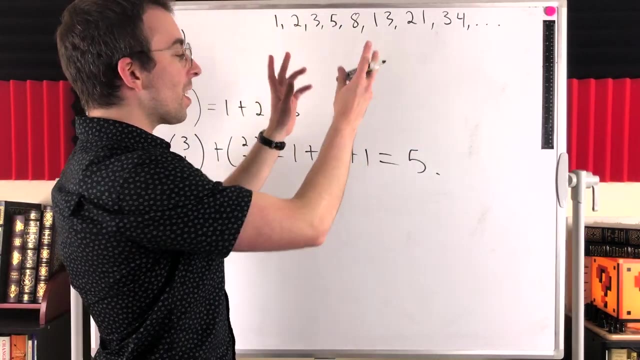 or, excuse me, the next few terms in this sequence are pretty cool. the next term happens to be 8, the term after that is 13, the term after that happens to be 21 and then 34, and they continue in this way. now i certainly encourage you to fact check me on this claim about this sequence, you know? try. 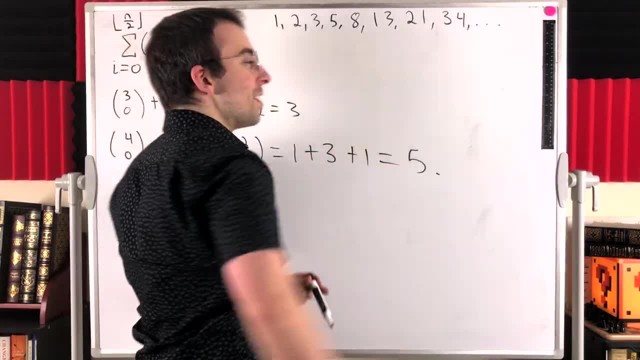 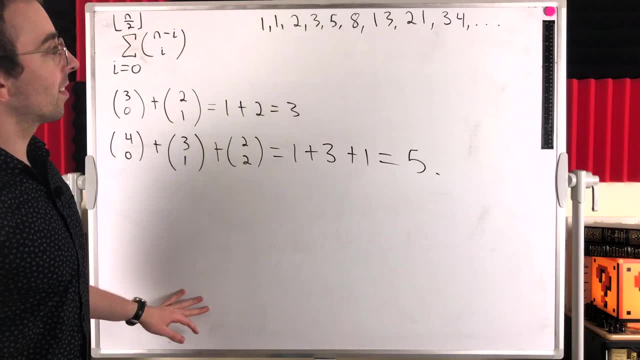 using our handy dandy formula that we explained. what are these numbers? do you recognize them? maybe you might recognize them if we place a 1 right at the start, just for kicks. those are the fibonacci numbers. what the heck are they doing here? who invited the fibonacci? 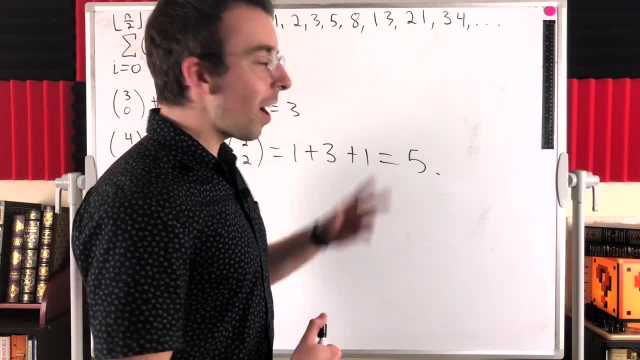 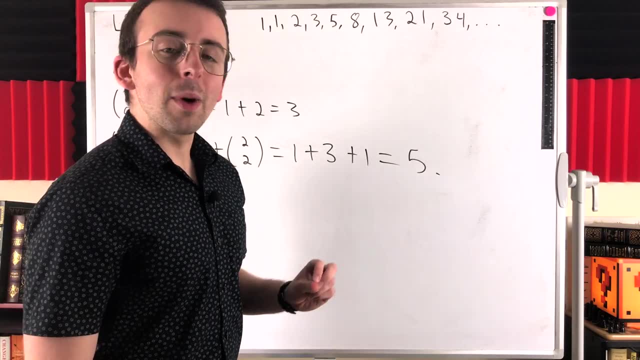 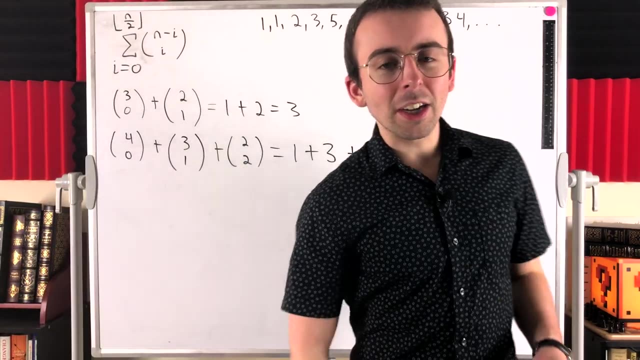 numbers to the party pretty neat, so why are they here? we'll talk about that in a future lesson. we'll basically just solve this problem again, but in a way that makes very clear why the fibonacci numbers are here. takes some time to think about it. let me know in the comments if you have an idea. 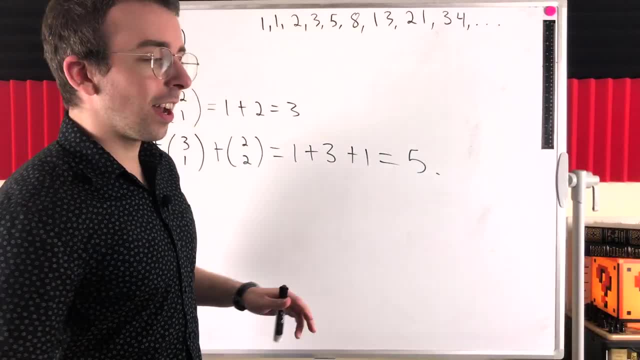 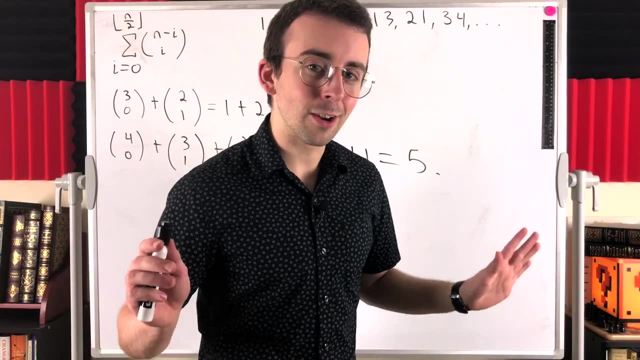 why we're seeing the fibonacci numbers here, and this isn't just an aberration or an aberration- i can't remember how that word is pronounced- this is going to continue to be the fibonacci sequence and it's a pretty clear why, once you realize what's going on. so i'll explain that in a future. 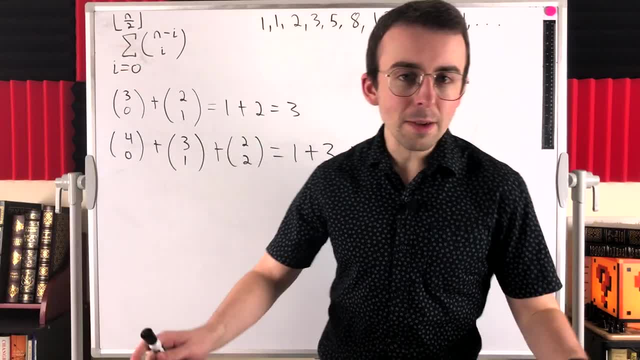 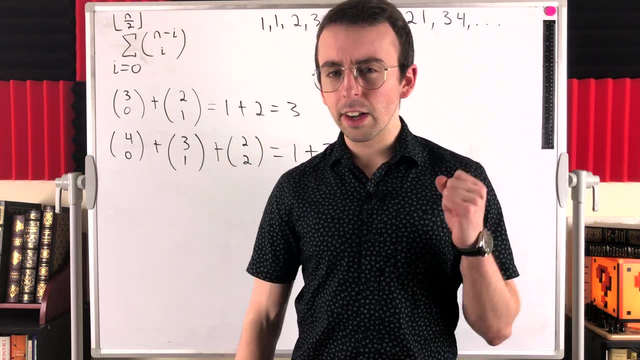 video. hope this video helped you understand how to count for any positive integer and the number of ways that we can write n as an ordered sum of ones and twos. let me know in the comments if you have any questions, need anything clarified or have any other video requests if you'd like to. 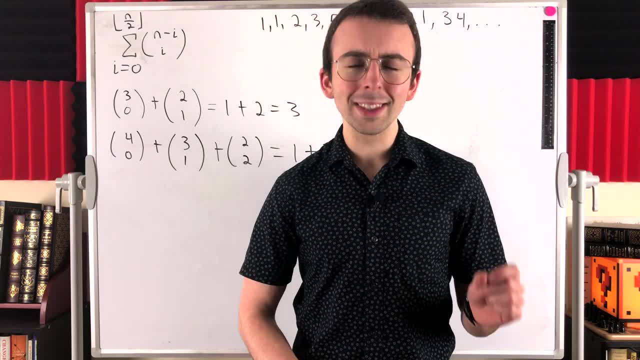 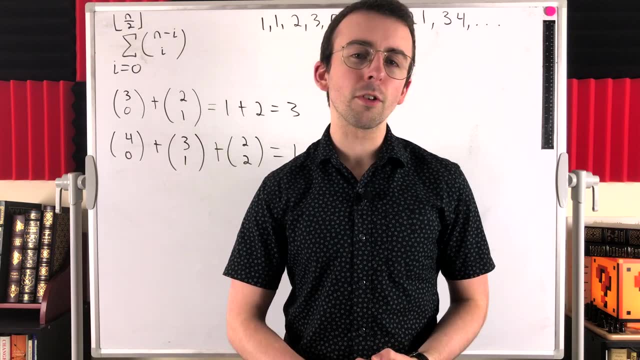 support the channel. i'd really appreciate a small donation on paypal or small monthly pledge on patreon. you can find links to those down in the description. thank you very much for watching. i'll see you next time and be sure to subscribe for the swankiest math lessons on the internet. you. 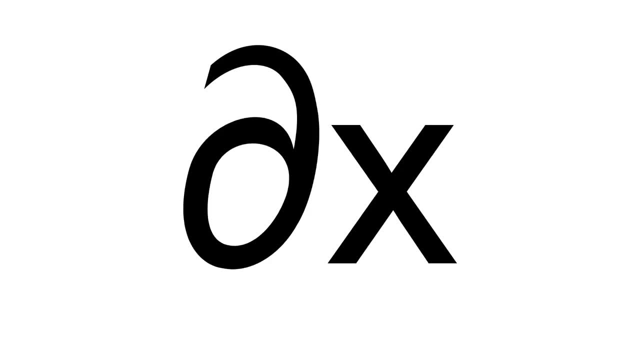 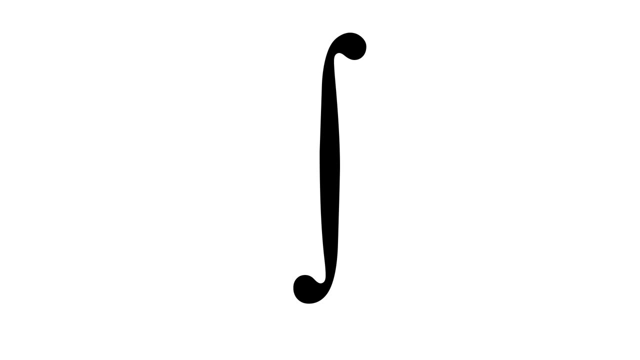 Change Really small. change Really small. change IT'S 3D: Add them up. Add them up, but like infinitely many times. Also, you can chain a bunch of these together and receive a proportional amount of tears from undergrads. 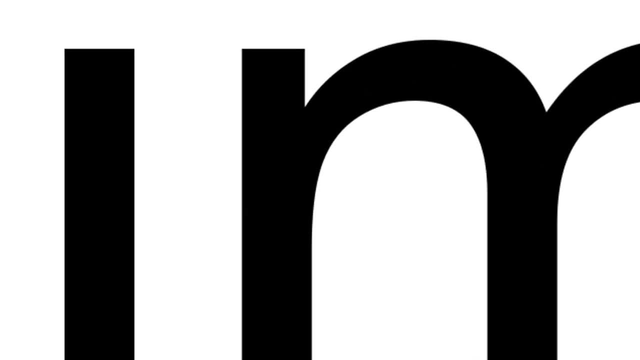 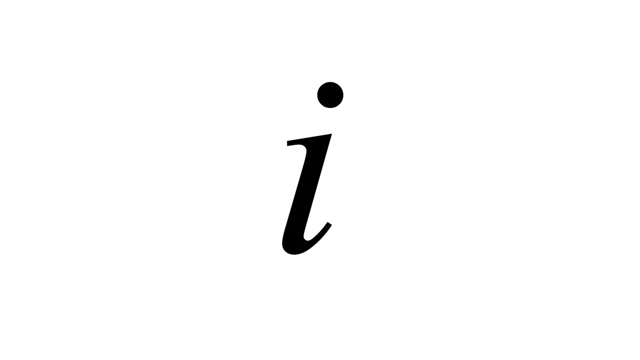 Hey, get closer, Closer, Closer. Okay, I can do this. Okay, I cannot do this. There's a penis joke here somewhere, Notoriously the most poorly named concept in math, right up until the tits group took its place.